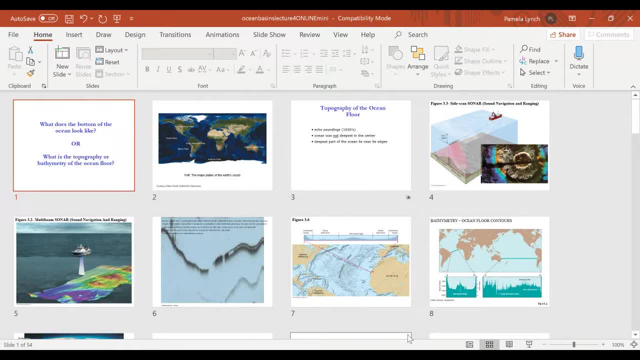 transform, being able to identify where those things are occurring on maps, knowing what's happening with the geologic events and the causes, It's a little bit hard to grasp. This lecture is now a physical and visible description and view of essentially what's happening as the 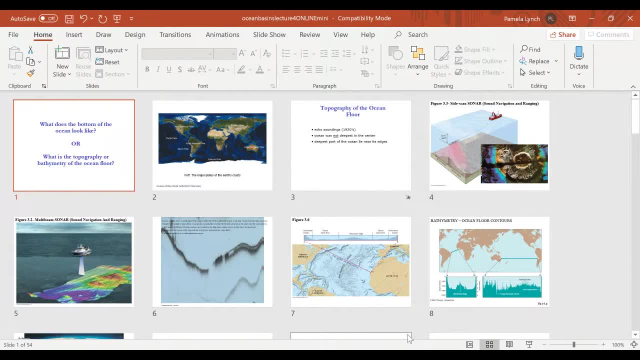 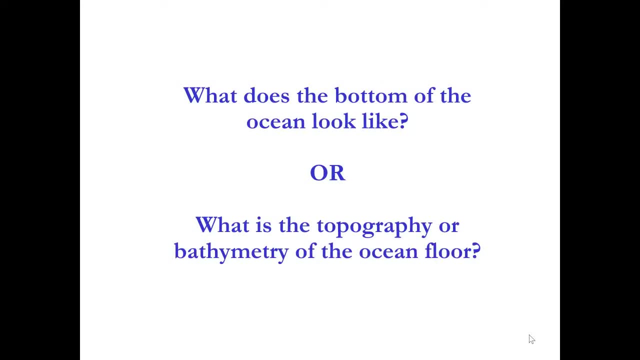 plate tectonic activities have occurred. So what's the remnants? what's left over? It begs us a couple of questions. Question one: if we know that seafloor spreading is happening in the middle of mid-ocean ridge systems, where plates meet, and we know therefore that the middle of 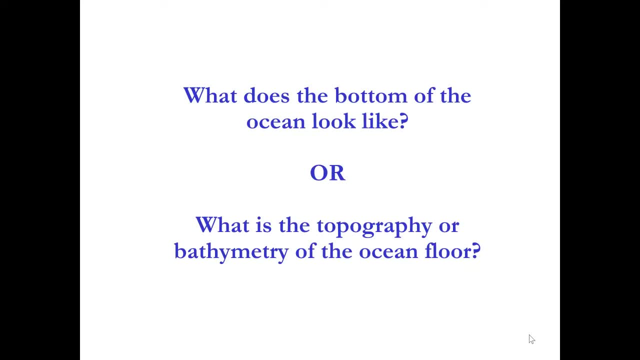 the mid-ocean ridge system is youngest and tallest and the edges are oldest and deepest. what exactly does the bottom of the ocean floor look like? More importantly, in putting with an oceanographic spin, what is the topography or bathymetry of the ocean floor that literally? 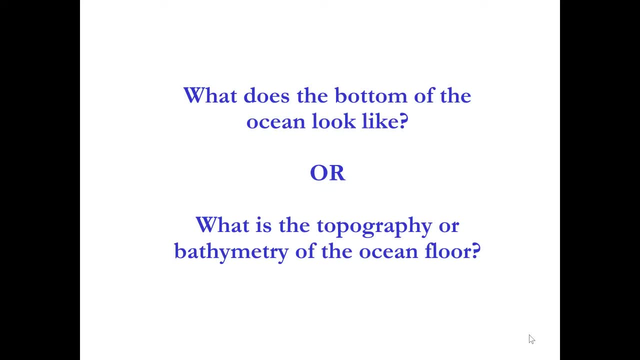 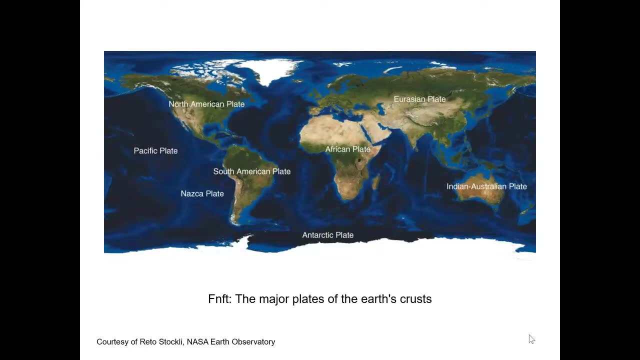 just means. what does it visibly look like if you were to draw a relief map, right with highs and lows, of what the ocean floor would be now? first things first, what you can notice. we've seen this, this figure, multiple times now. okay, the earth has eight major plates and eight minor plates. roughly 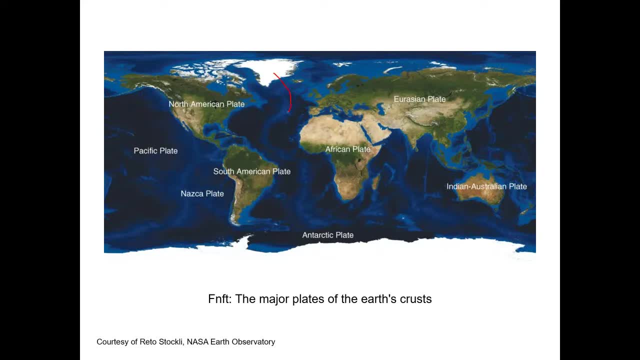 and when you look at a photo like this, you can see that there are shallow areas represented in blues. okay, those are along the coasts surrounding a lot of what we call the continents, but they're also along the mid-ocean ridge systems. there's one in the pacific, okay, so we know, of course, that. 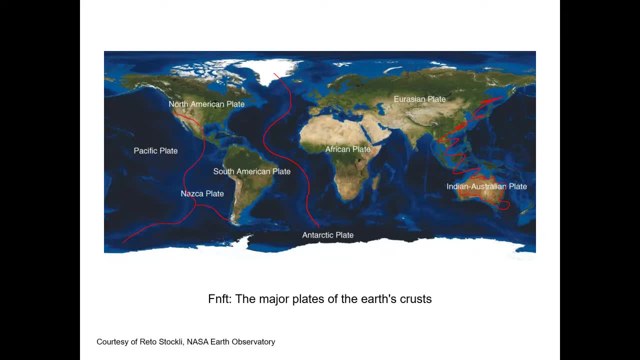 those lines that i've just drawn are going to be your shallower zones. for example, in the atlantic mid-ocean ridge it's youngest in the middle and shallowest in the middle. then these dark blue areas are representing where it's deeper. we also know that that also means not. 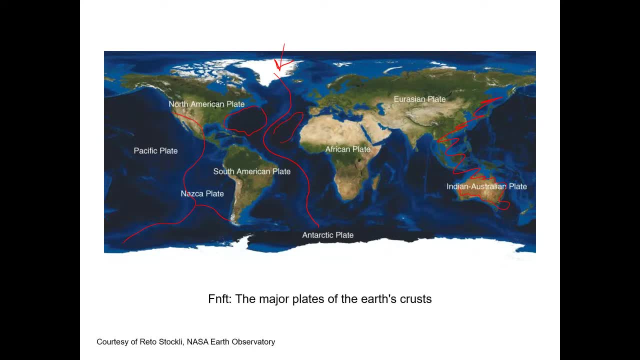 only is it deeper, but it's older. okay, so if we were to drain this picture of all the blue and literally just have our plates, we'd have our continental crust and our oceanic crust exposed again. oceanic crust would be here here. newly formed ocean crust would be here. 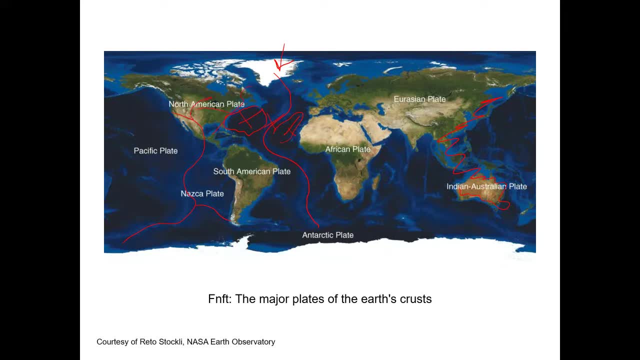 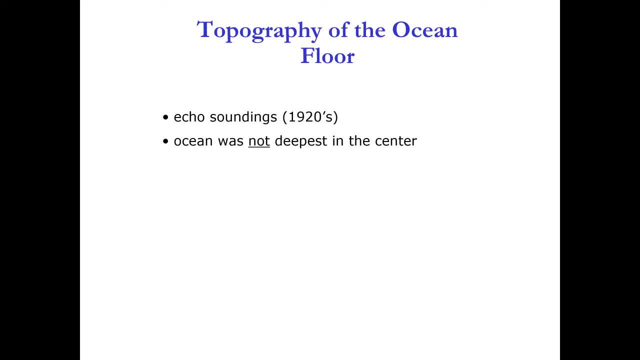 continental crust starts there. okay, so if we drain that, what's it going to look like? well, we didn't know right at first, so we started off with doing echo soundings, which is essentially bouncing sound off of particular beams that go through the depth of the water and they hit and stop, essentially, and then you can read a relief. 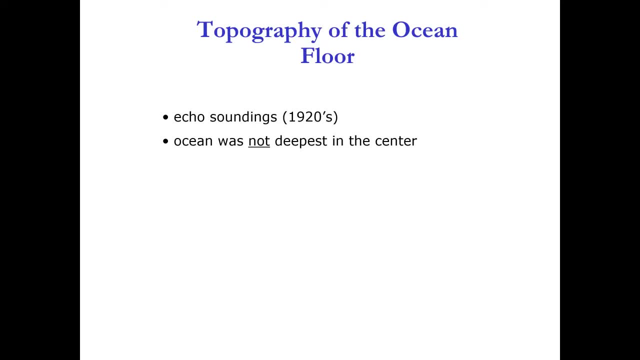 or reverse map. it confirmed, of course, what we knew from plate tectonics: that the ocean was not deepest in the center, because, again, that's where the mid-ocean ridge is- shallow there- and that the deepest part of the ocean did in fact lie at the edges. so here's a visual. 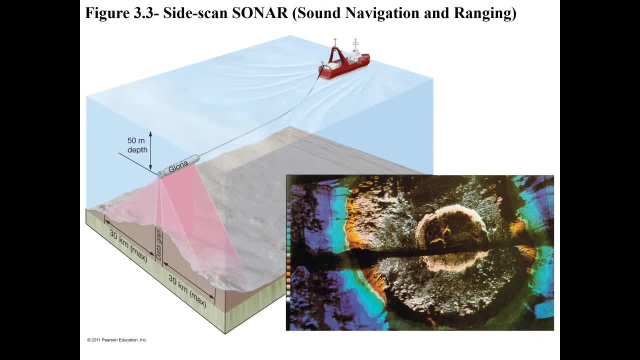 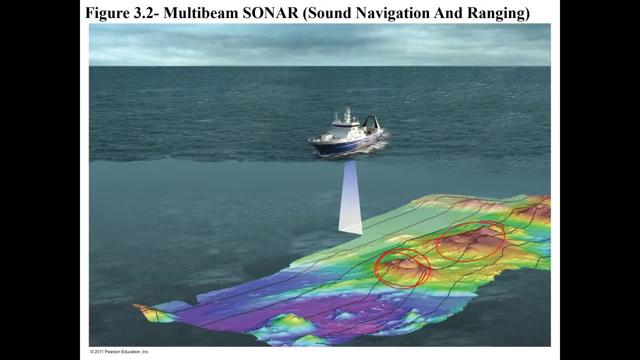 explaining how sonar works, how echo soundings work and giving you what those relief maps look like. so now you can see that there are higher points, which again would be shallower in an ocean, and lower points which would be deeper in ocean. now this is pretty and easy for you to see what 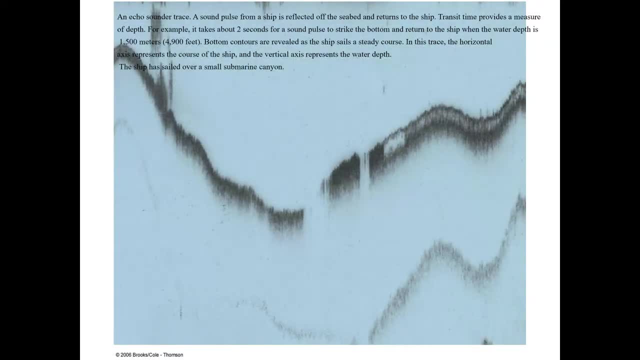 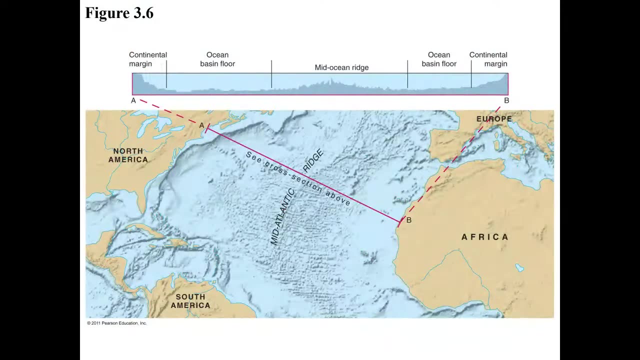 actually comes out on the boat are soundings like this. but what it does matter, what is it? tells you deep and shallow locations. why do we need to do this? well, it's important to map the sea floor one so that we can find cool biological areas like hydrothermal vents. 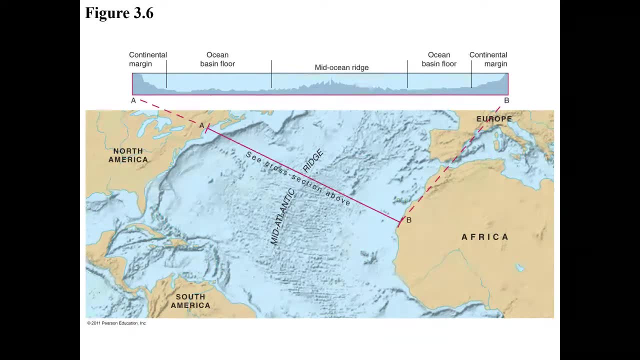 which you'll hear about at the end of this lecture. it's also important because it does impact currents and it impacts how the ocean systems are moving and if it's really shallow, of course it would really matter if you were a boat and you need to know what's underneath you from a biological 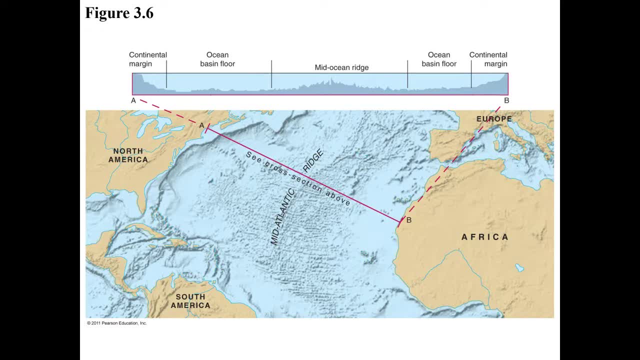 perspective. also, it can influence where fishing grounds are and how migration paths of a lot of transmigratory fish, like sharks, may travel. so what they've done is given you an example of a transect from the north american plate- there's the edge, okay- to the african plate. 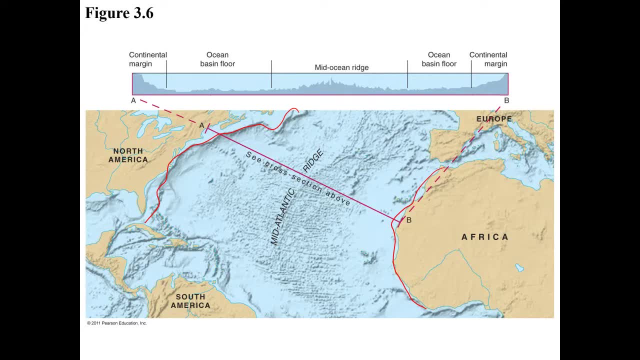 and there's the edge, okay. and they transect, of course, through deeper and older sections and shallower and younger sections, and that translates exactly to this figure up above. so here's our middle, our mid-ocean ridge. sure enough, it is shallower there, the edges match up with the deeper ocean basin and then we hit back up on land again. 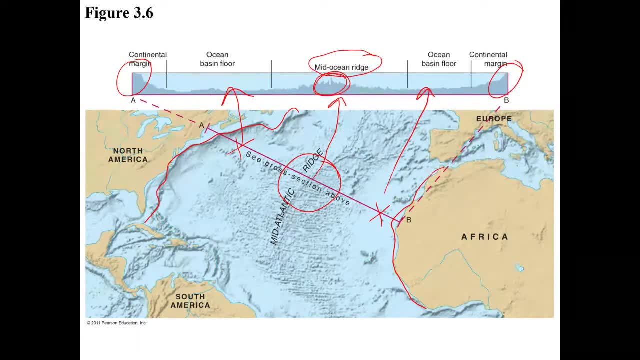 you're going to then be mapping this type of figure in lab four and you're going to do one map for the atlantic ocean and a series of maps for the pacific ocean and you'll be labeled, labeling them as such. you'll label the mid-ocean ridge, you'll label the margins or the sides. 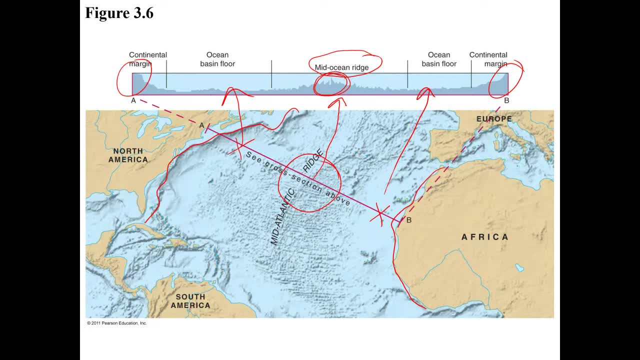 and you'll label the ocean basin. what this lecture is going to do now is focus specifically on what does it really look like? okay, so right now we have a bunch of dots and high and low points, but what physically is there? so we're going to look at what happened in the ocean basin floor. 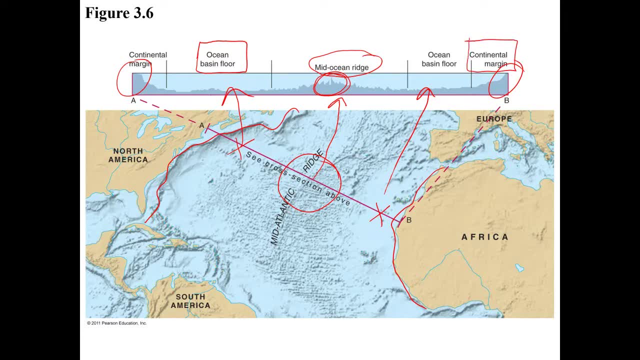 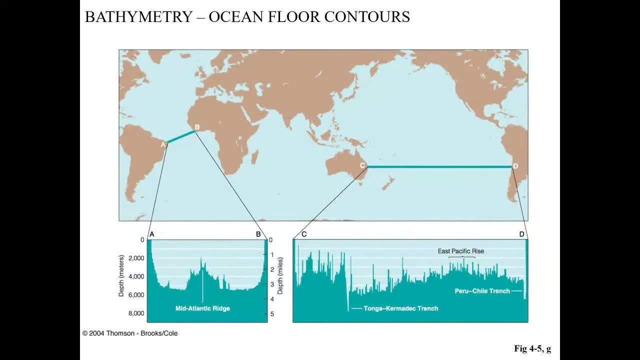 and we're going to look at what's different and happens in a continental margin. you'll notice that continental margins, like the margins on a paper, are on either side. okay, so just one more example before we start getting into some of the definitions and nitty-gritty of this stuff. i want you to realize that you're going to be doing an 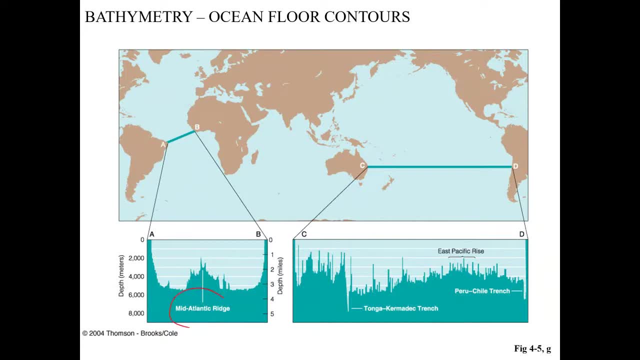 atlantic ocean transect- okay, here it is- and a pacific ocean transect. notice, there's a massive difference. you see no mid-ocean ridge here in the pacific example. instead, you see some things that are indicative of. think about it. from plate tectonics, what are trenches indicative of? 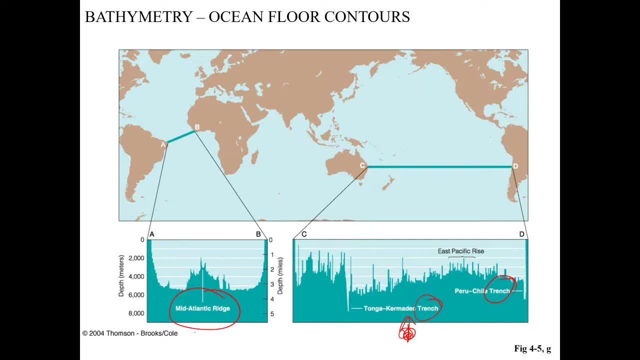 subduction or convergence. so here you have sea floor spreading and a divergent plate boundary. so that's represented, of course, off the coast of north america and off the coast of south america. and if you leave off the west coast of north america or off the west coast of south america, you have an entirely different type of plate tectonics. 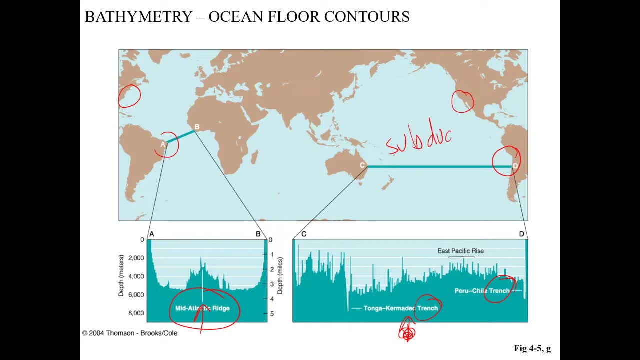 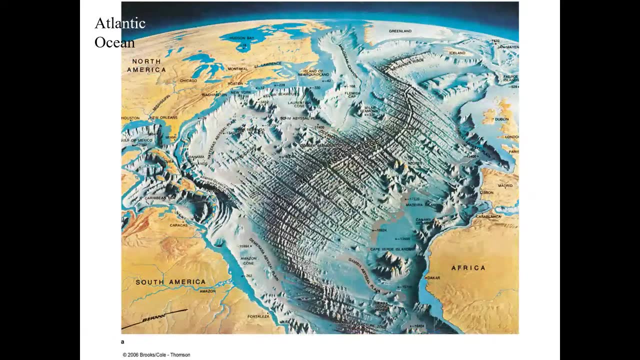 you then have subduction instead. so of course the relief maps or the bathymetric maps should look different, and of course they do. this is one of my favorite pictures. i actually have a picture of this hung up in my office because i think it's so beautiful, but it shows what i call the backbone, or 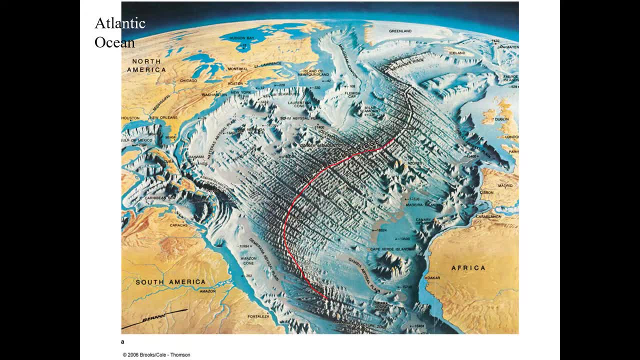 the zipper, which is our mid-ocean ridge, and here's the center of the mid-ocean ridge. remember, it's never a straight line. why? because it's separated regularly by faults, right where things are going to slide laterally, just like a sliding glass door. but it does in fact show you that there's. 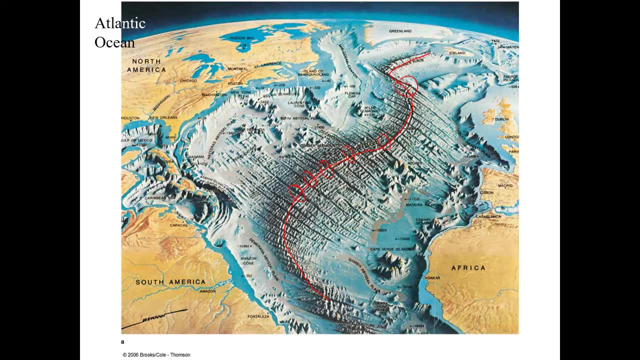 a mountain in the middle of the ocean. that mountain is called the mid-ocean ridge. on either side of it it gets deeper and older until, of course, you hit continental crust, as you get to what we call the parts of the plates that you can see flying overhead in an airplane. okay, 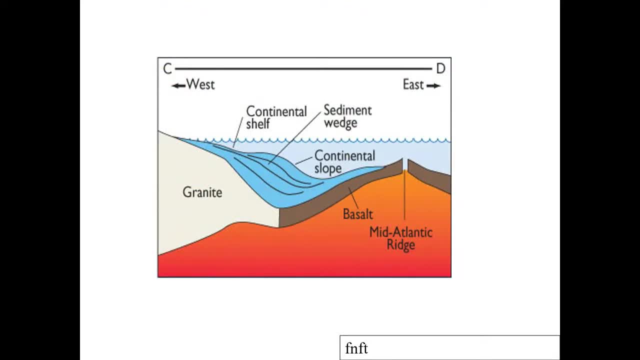 so let's make sure we understand where we are in this lecture in relation to the lecture that we just covered with plate tectonics. okay, so here's our mid-ocean ridge system. this is representing divergence, right? we know that. that's seafloor spreading. what's happening there? the basalt that is in 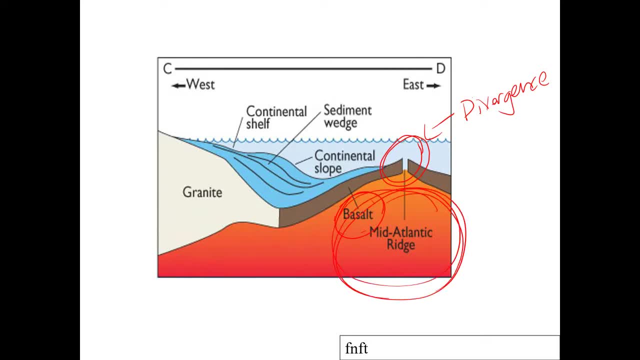 the asthenosphere. so here's where the convection current of the extenosphere would be- can push through this area, causing the divergence or the separating of oceanic crust. that oceanic crust will form new in the middle. so that's so pushing this apart. remember those. 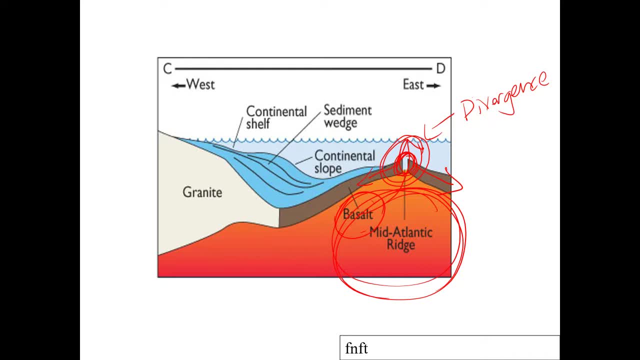 are stages one through three of the wilson cycle. that means that this entire plate right is shifting to the left, it is being pushed up and out of the way. why? because this is basalt, an oceanic crust, and this is granite, which means continental crust. there are two densities: granite: 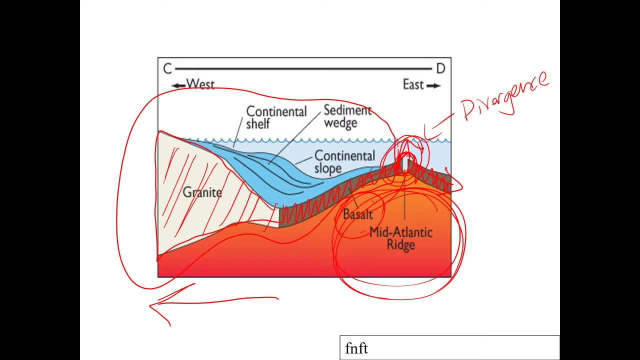 is less dense, so it gets pushed up and out of the way. it then becomes the edge of the continent or located in the middle and the area of the continent. so this is a very interesting offered portion here of the edge of the continent and there are these hedges right here between two. 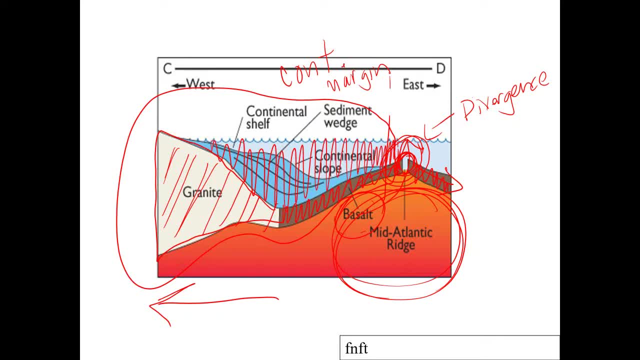 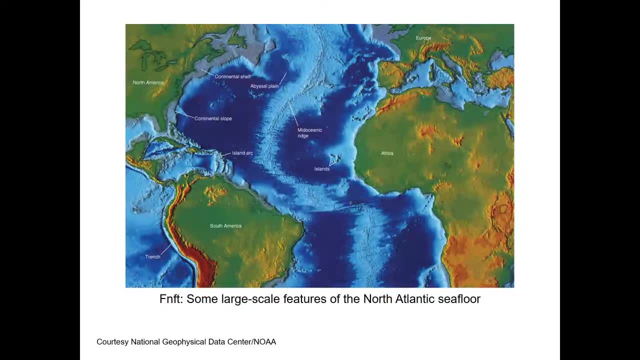 nodes, and this is an idea that's working with this particular one here. it is making a dike of just natural dunes that are still floating there, so let's start with this one. so the dike is the area of the continent, so this is the edge of the continent, so there is a space. 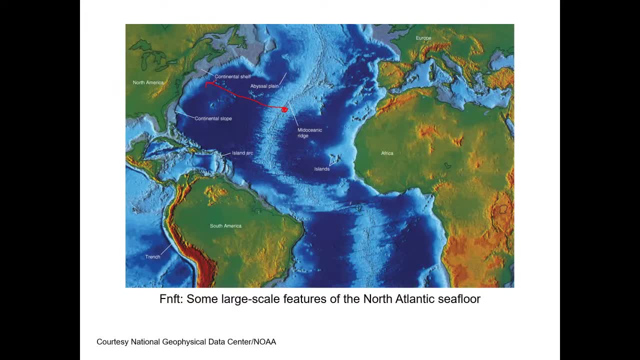 of qoran in the middle of that section, and it is not a very long space, but it's going to be longer than a hundred hundred feet. so this is where we're going to call the edge, a margin. so the continental margin is made up of a series of locations. again, the water is filling over that section. 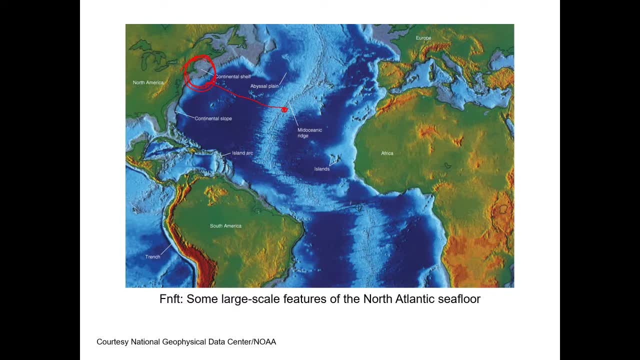 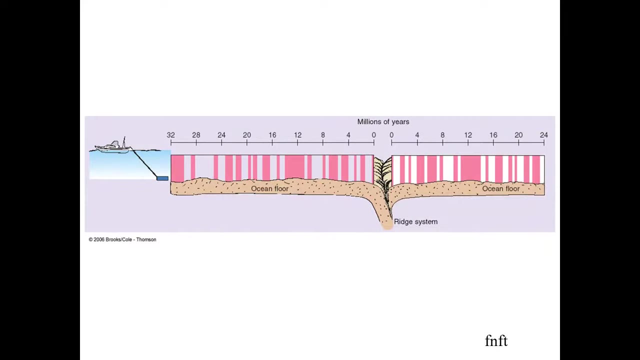 a change in topography, change in coloration. you know you have a margin and the margin is a shelf, a break, a slope and rise. the rise is the location where it meets the deep ocean floor and allows for sediment to build. we know these things are true because, again, the echo soundings have shown us. 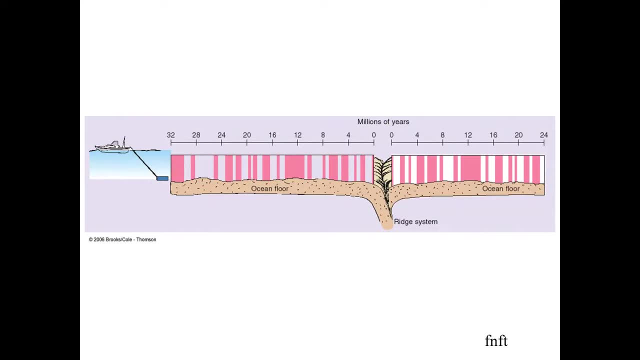 that, and it happens over millions of years. again, think back to the lecture before this. how many millions of years can this boat travel until it gets to the edge of an ocean? hopefully you said the date was pangea, right, so about 200 million years ago. so 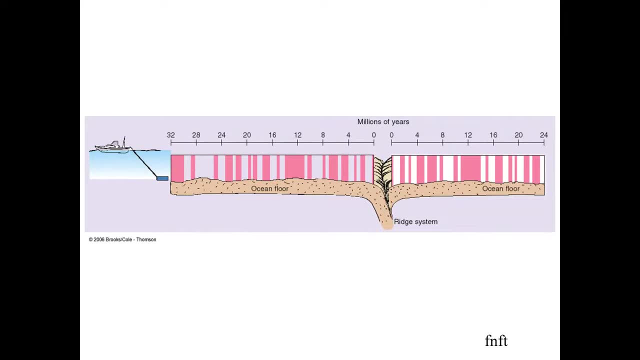 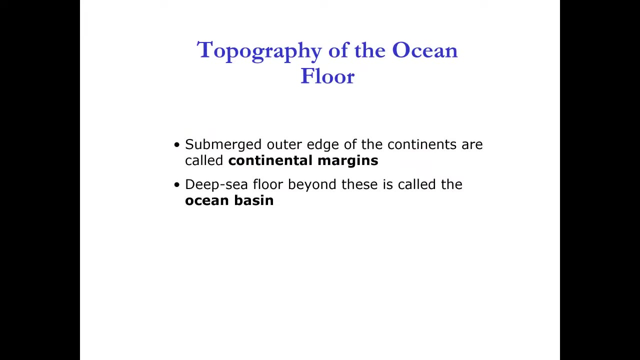 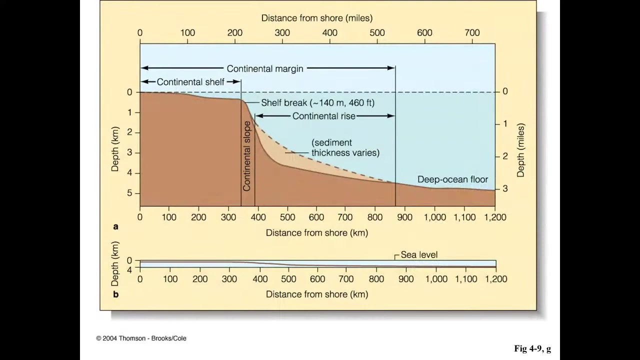 this boat in this example, has a lot more space to travel. so if the topography of the ocean floor is going to cover two components- the continental margins in the ocean basin- what we're really doing is showing that this is the continental crust- again granite, which is less dense, and this is the oceanic crust, which is basalt and that's more dense. so here we. 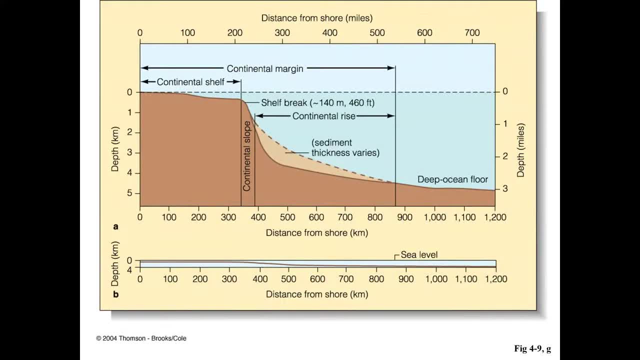 go. this is your classic figure for this particular lecture. this is the figure that you should spend the most time with. go back to it, study it, memorize it, work with it. use it when you're doing your quizzes, use it when you're doing your work, use it when you're doing your labs. it's the perfect figure. 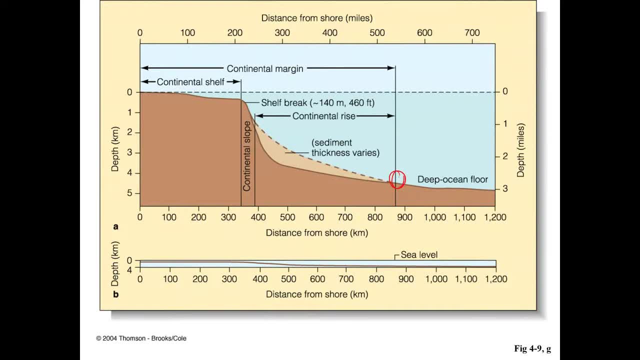 exactly what's happening when the ocean floor meets- or the ocean floor, remember, is oceanic crust- when the ocean floor meets the continent, when it meets the continental crust. so take a look where this continental margin is extending from, from the area where you would lay your towel. 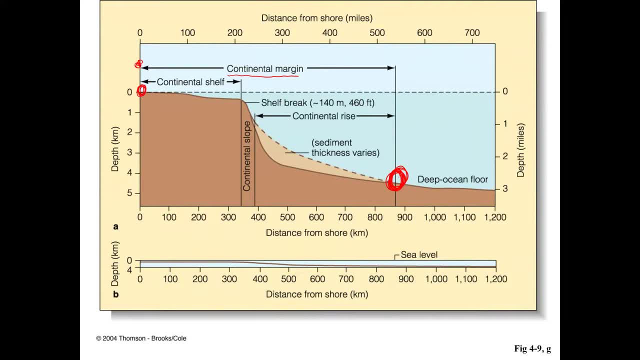 okay, literally where water meets, land to the edge of where the ocean floor meets. in other words, every thing here is granite and everything here is basalt. so stuff that you would find in the deep ocean floor is going to be different topographically than the stuff you're going to find. 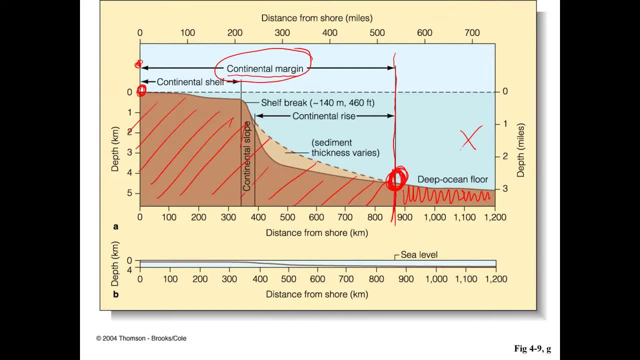 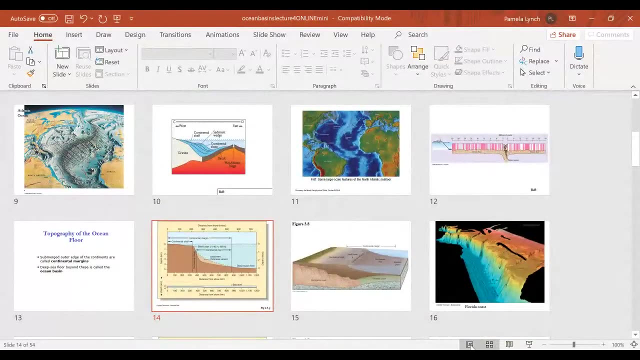 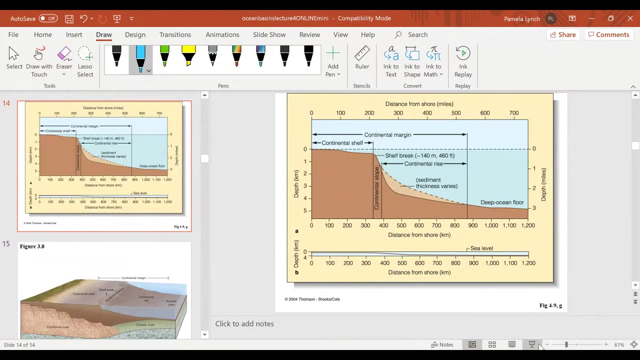 in the continental margin. so the margin has four components. okay, they go in order from closest to shore to furthest from shore. they're just going to change the color, open it back up again, change the color of my drawing. okay, they go from shallowest to deepest or closest to shore to furthest. 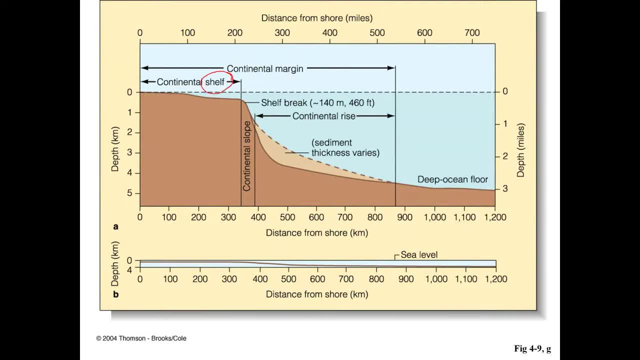 offshore. they are the shelf, the break the slope and the rise. again, shelf, break, slope and rise. they go in that order. by definition, the continental shelf is a submerged, shallow extension of the continent. again, what you can see here is that it is at, or just slightly below sea level- okay, zero, essentially kilometers- and then gets slightly. 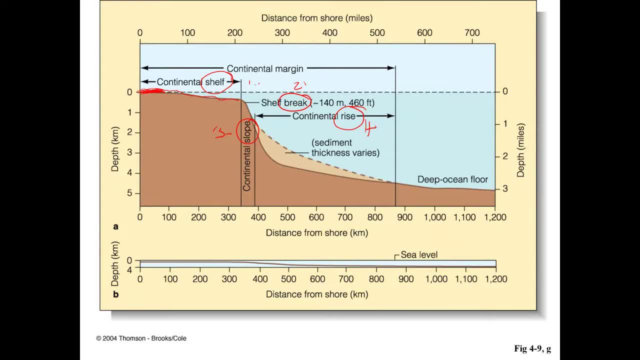 shallower. that's a shelf. you could lay a plate on here right or ride your bike and you still have to pedal a little bit. can you hit a spot where, if you were riding a bike or rolling a ball, you literally would stop pedaling and you would just have a free fall? it's a hill. that hill, of course, is called a. 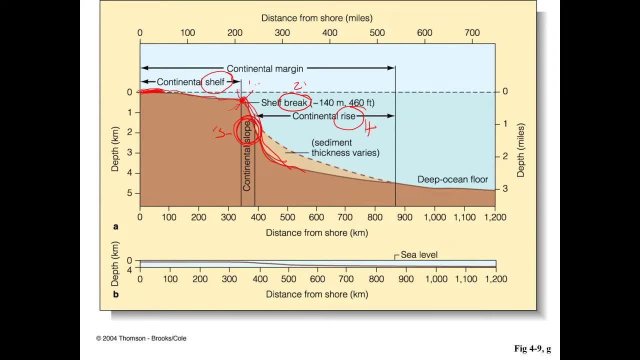 slope. okay, at the exact meeting point of where the shelf meets the slope, we call that the break. that's the place where you go from the submerged, shallow extension of the continent to the actual hill. the final component here is the erosion or the sediment mound. this is on top of the actual 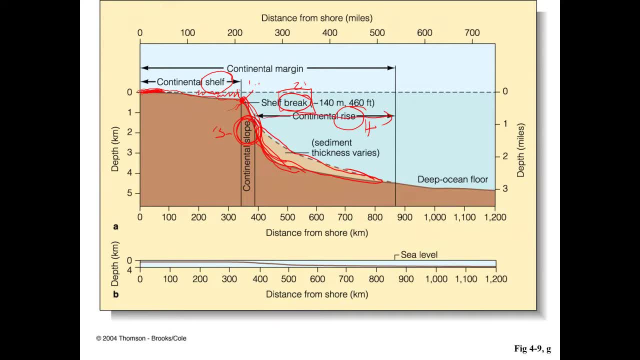 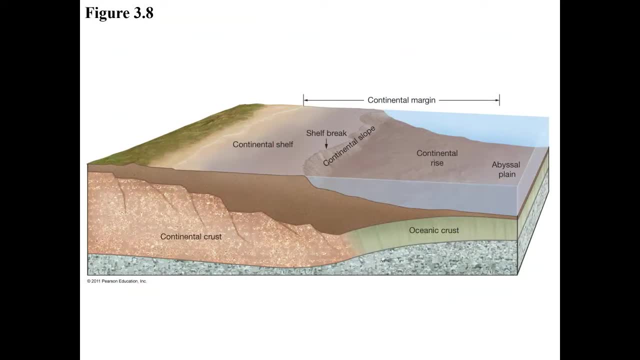 and connected to the actual slope and continues up until we change from granite to basalt. you'll be labeling all of these things in your atlantic ocean figure for lab 4, so again, you're going to have them on both sides of that map. here's another figure that i think equally shows. 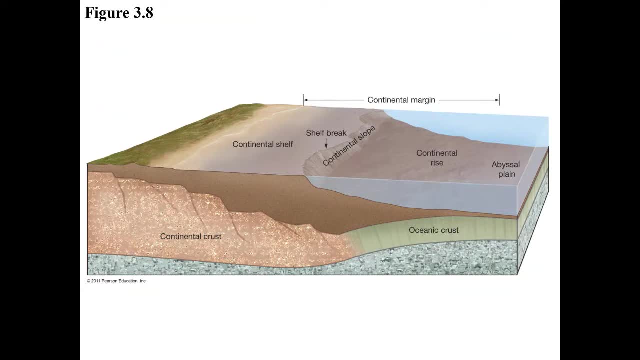 you a great perspective. here's another figure that i think equally shows you a great perspective of how these four components are. remember the entire thing is called the continental margin. a margin means edge, so this is the edge of where the continental crust meets the oceanic crust. 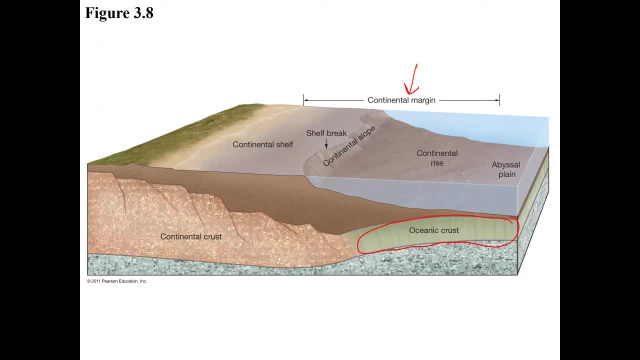 the oceanic crust is more dense, so it's pushed down. continental crust: less dense, so it's pushed up. okay, so this is what's under the water in the deeper portion. this is what's under the water in the shallower portion and then literally above sea level at the 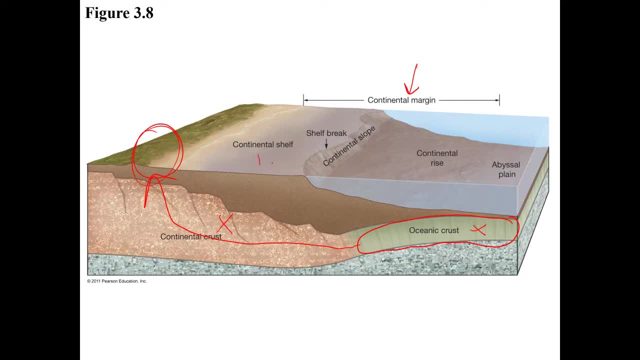 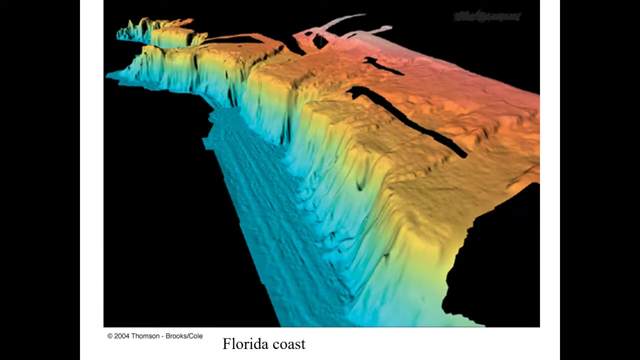 entire margin has four parts: shelf, break, slope and rise. once you get past the rise, you're in exclusively oceanic crust. see how, where the margin ended. so this is your ocean basin. okay, here's a physical, pretty beautiful image, i believe, of the florida coast. so here's your. 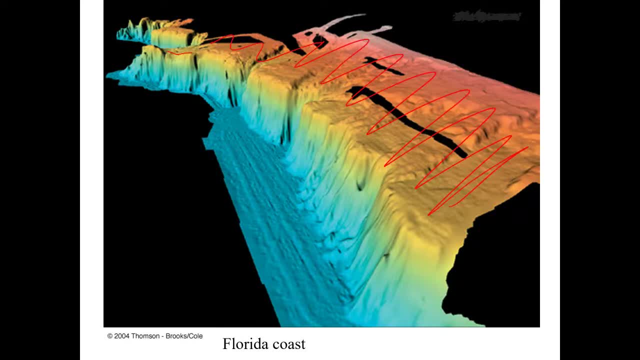 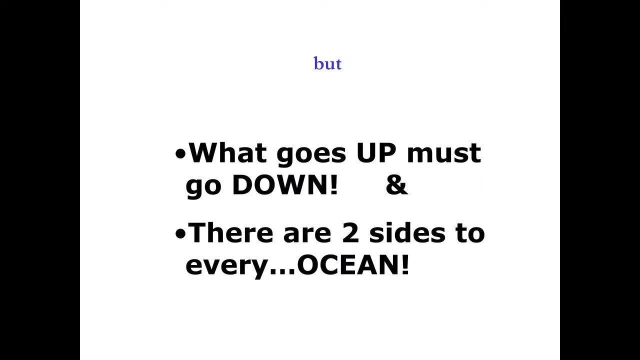 shelf. that is your break, that's your slope and that's your rise, so that's where the erosion is. anything past here, of course, is going to be deep ocean basin. remember, though, if we've gone down on one side of a plate and then met at the middle of a mid-ocean ridge, this must, of course, happen on a flat surface. 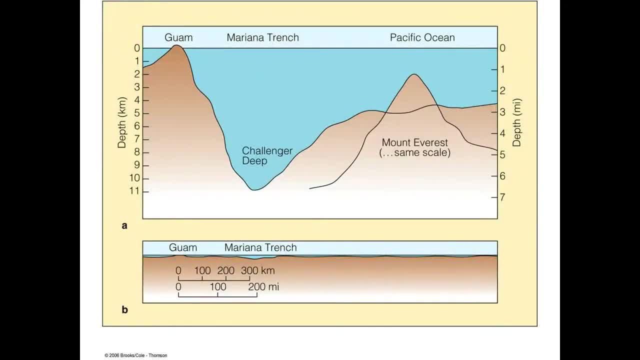 the other side. so what goes up must go down. because if you think back to plate tectonics, we need isostatic equilibrium. everything has to balance. so where there's a deep there's a tall. so of course, from a plate tectonics perspective, if you have a margin on one side, 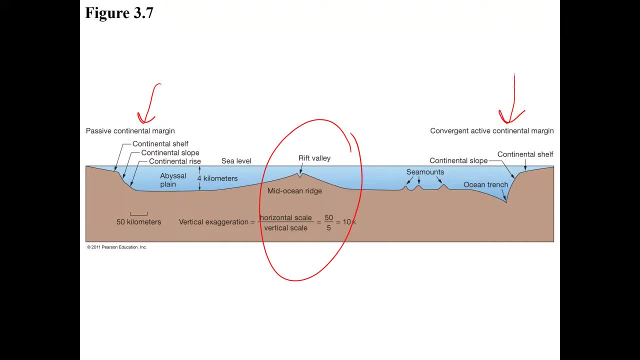 and a mid ocean ridge in the middle. you should have a margin on the other side. so notice, you have two margins, just like on paper, two edges right, two one inch margins, or half inch, whatever you said it has. so it's showing you that you have a middle aptly named the mid-ocean ridge. 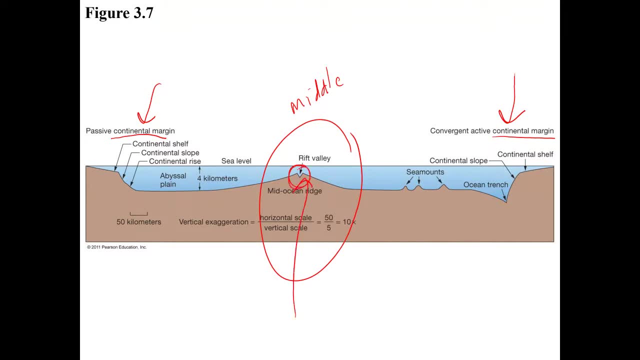 in the middle. what is happening to form this rift valley? what is happening to form that mid-ocean ridge divergence? okay, so we know that so far seafloor spreading is occurring there, and then we know that it's young and shallow and it has to get deeper in the ocean basin as you go to the left. 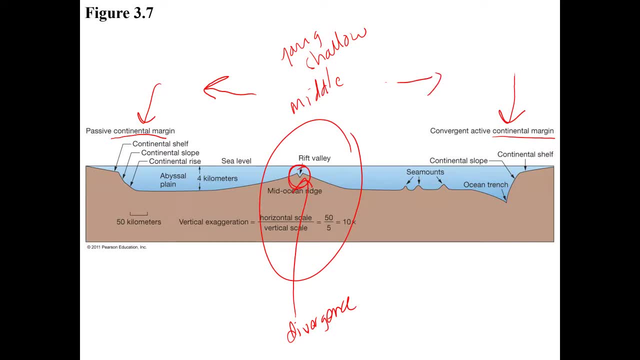 and to the right, but it only gets deeper until you hit your margin. so there's the margin on the left and there's my margin on the right. notice that the margins are not the same distance from the middle and they don't have the same topographic features. on this side you just have an abyssal plane which is sort of a flat. 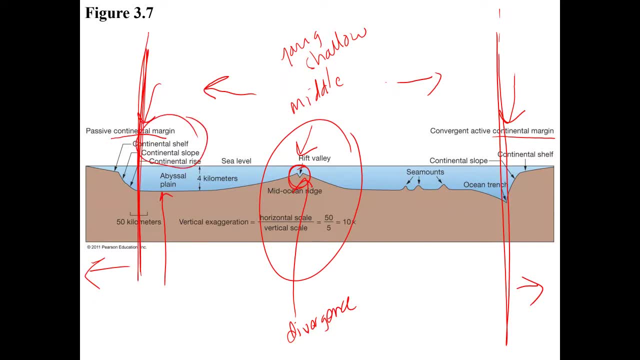 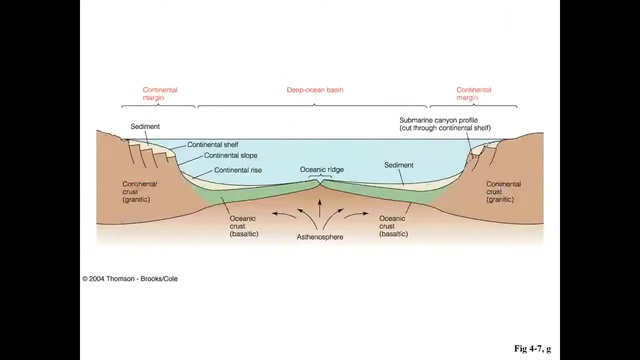 featureless area and again your four components of the margin. on this side you have things that are indicative of subduction. so over here is convergence. okay, we still have our margin examples, but they're much steeper and they end at an actual trench. another visual showing you the same thing: on this particular side we have flat featureless. 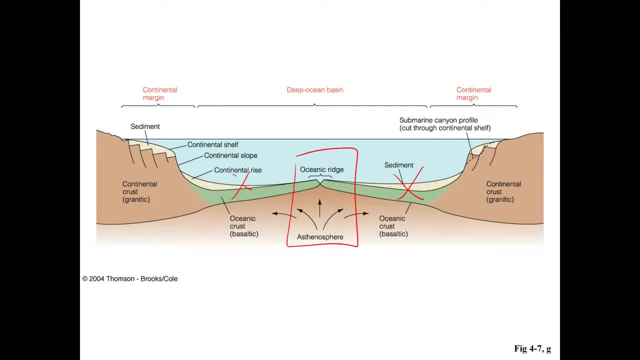 rises on both sides, opening up from the mid-ocean ridge system. so this is a divergence, only example. okay, what it's showing us, of course, is a margin on either side, giving us our shelf, our break, our slope and our rise. our shelf, our break, our slope and our rise- mid-ocean basin, exclusively in the middle. 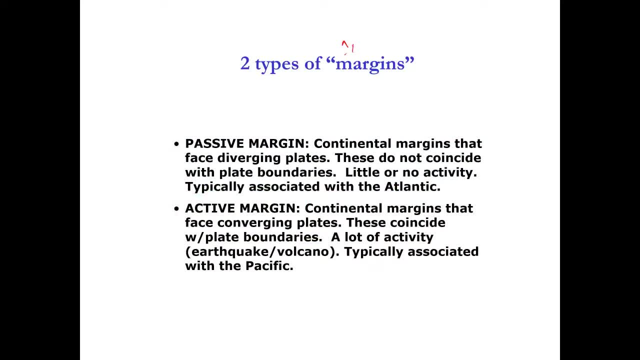 now we've talked about the word margin, right, and we've called it a continental margin. there's actually two types of margins: passive margin and active margin, and these literally match up with which type of plate boundary it's lowering each time, changing place for eachreet boundary, etc. 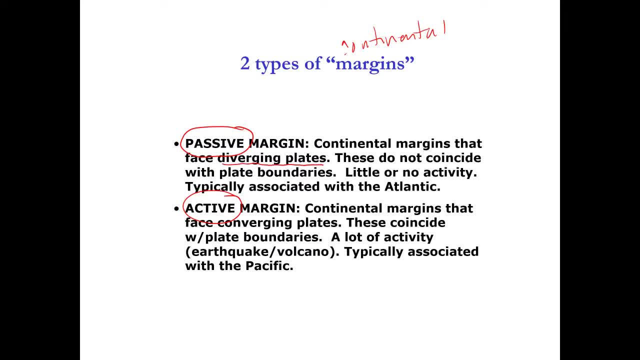 by Passive margins match divergent plate boundaries and active margins face convergent plate boundaries. So a convergent plate boundary is going to be where there's a lot of activity because you're close to a subduction zone. In a passive margin there's not a lot of activity because you're near just. 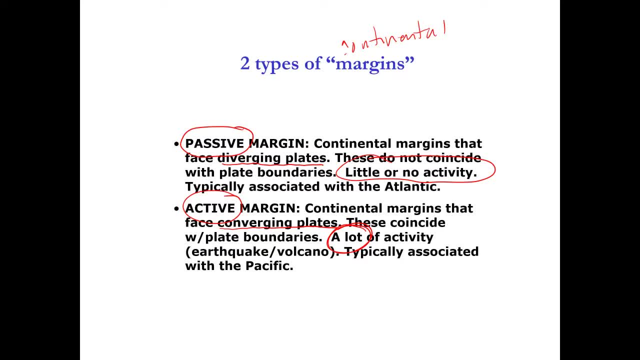 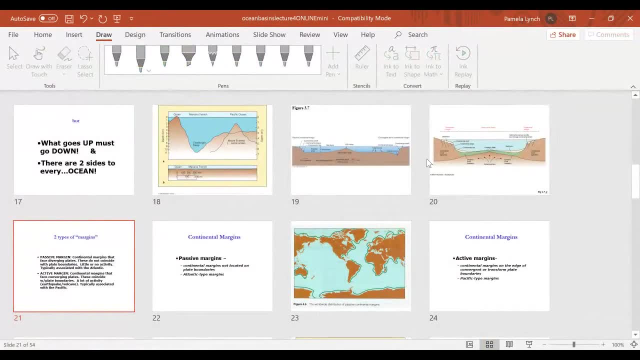 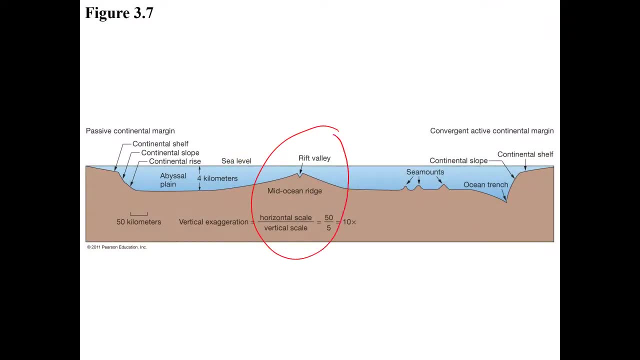 seafloor spreading newly created seafloor. I'm going to go back to the figure that we just saw and remind us one more time of these margin types. So here we are. there's our mid-ocean ridge system. This means this is divergence right. This? 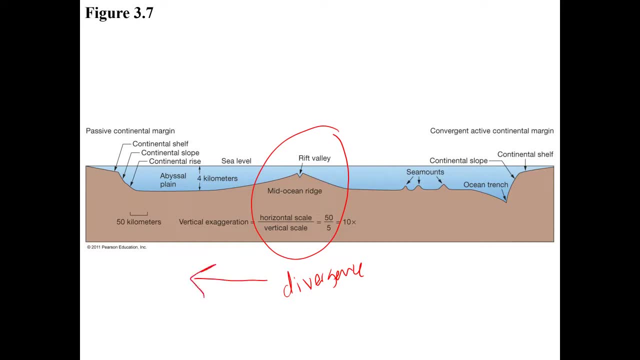 divergence is causing this plate to shift and move to the left on this side and it pushes up the continental crust on this side. Because it's facing a divergent plate boundary and it's far away from the mid-ocean boundary, it's not going to be able to push up the continental crust on this side because it's facing a divergent plate boundary and it's far away from the mid-ocean. 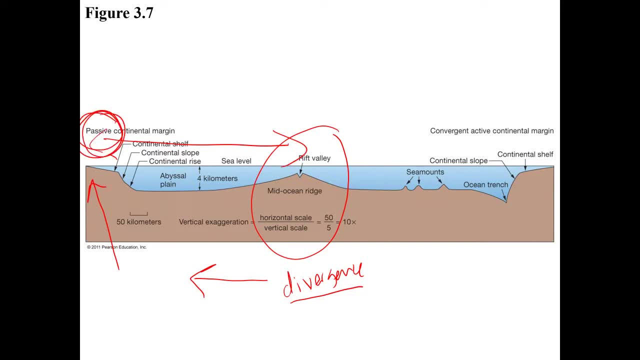 boundary and it's far away from the mid-ocean system. It's a passive continental margin. Now, over here, you still have divergence. right, Divergence is here, But before you get to the margin on this side, what did you get? Convergence. So of course, this side has to be an active 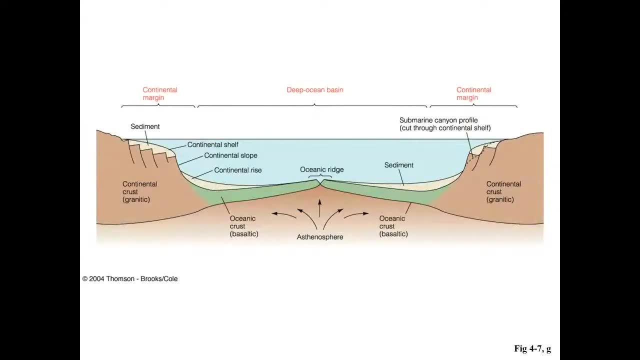 margin. In the next example, we literally have only a mid-ocean ridge system. okay, only divergence. So this side has to be an active margin. In the next example, we literally have only a mid-ocean ridge system. okay, only divergence. So this: 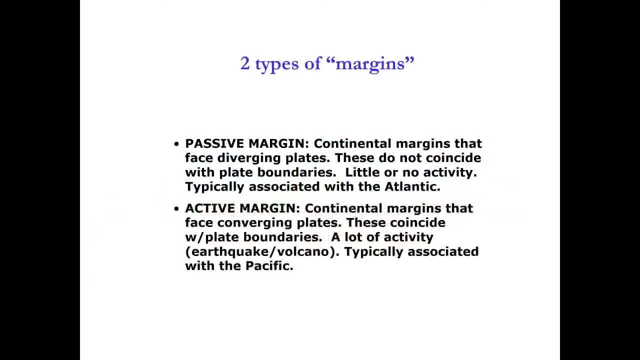 side has to be an active margin. In the next example, we literally have only a mid-ocean ridge system. okay, only divergence. So this is passive and this is passive. What you do, of course, is you interpret the boundaries to figure out where you would have active and passive margins. So 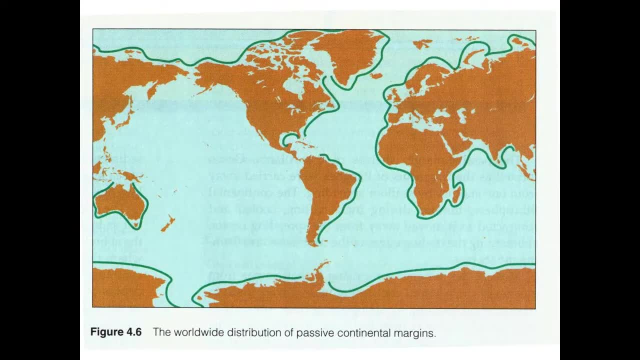 here's a figure of the United States in the center, there, with the rest of the Earth and all of the land masses. It's our seven continents. and we're not looking at a plate map right now. we're looking at as you fly overhead in an 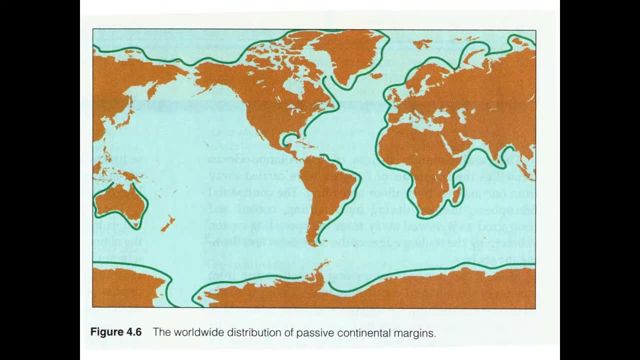 airplane, where the continents and all the land masses are that stick up above water, And anywhere that you see a green line is telling you that it is a passive margin. And anywhere that you see a green line is telling you that it is a passive margin. 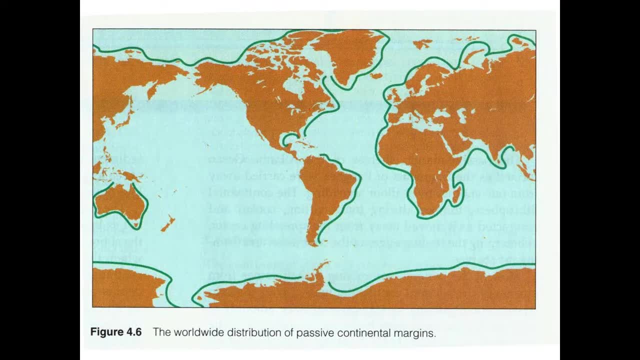 So let's make sure that this makes sense. Okay, here we are. okay, east coast of the United States, We know that our mid-ocean ridge system is right in the center of the Atlantic Ocean. So if this is a divergent boundary right here, then you better have a passive. 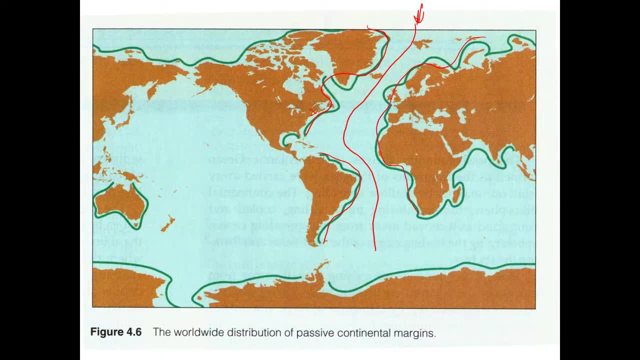 margin on either side, which makes sense. Okay. over here, though, you have a convergent margin, So if this is a divergent plate boundary along with a whole series of trenches, that let us know that convergent boundary is there, along also with a. 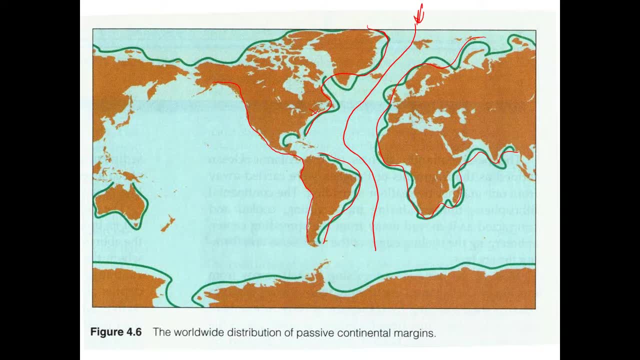 series of fault lines and because of that you don't see any green. So this over here is an active margin. Passive margins here, all along the Arctic as well, and surrounding Australia. Everywhere else is an active boundary. Active margins, of course, are the ones that we're looking at here. 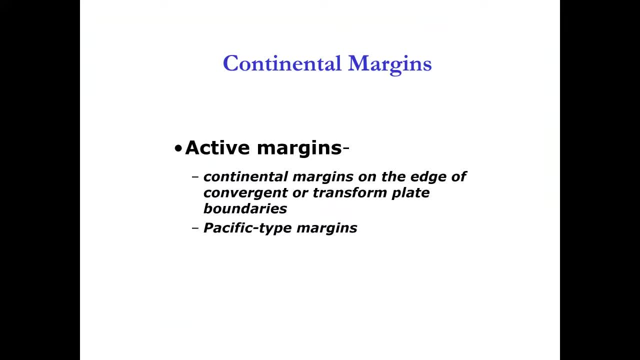 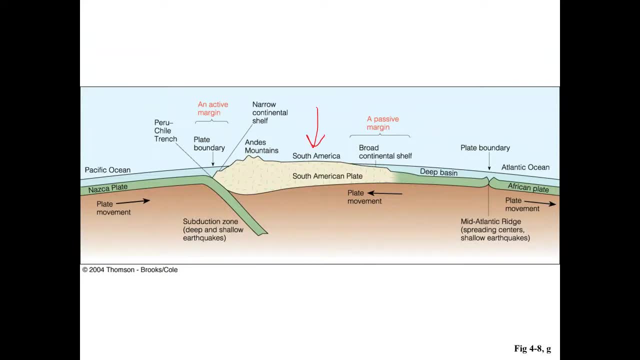 So if you were to look at an example, this is the South American plate, but it could equally be the North American plate. It's the same answer. okay, You were to turn it on its side and look at the west coast versus the east coast? Okay, 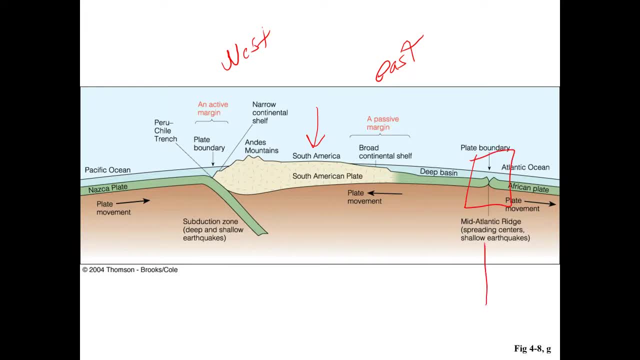 I have a trans-designed Tipper plate right here. So if you were to have the MAS here, you would see that it would often be an active lacked margin, And then again you really have to have a peep on it. And on the east coast, what do you see? A mid-ocean ridge system. 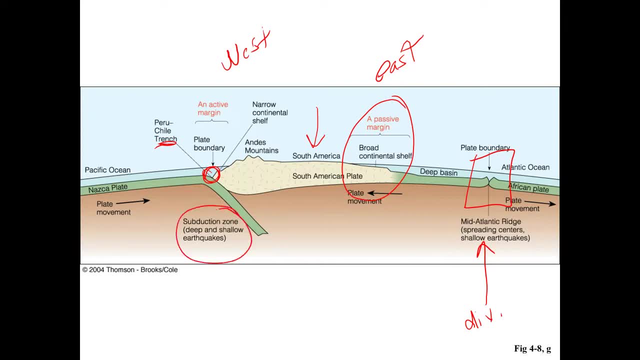 telling us exclusively that this is divergent. If this is divergent, then this side of the plate must be a passive margin. Conversely, on this side, what do you see? A trench. That trench is telling us that it's a subduction zone or a convergent boundary. That means that this plate, the nasca plate, is actually subducting underneath the South American plate. It's gonna draw in all the layers of the plate, literally. right, there are two planes In this. 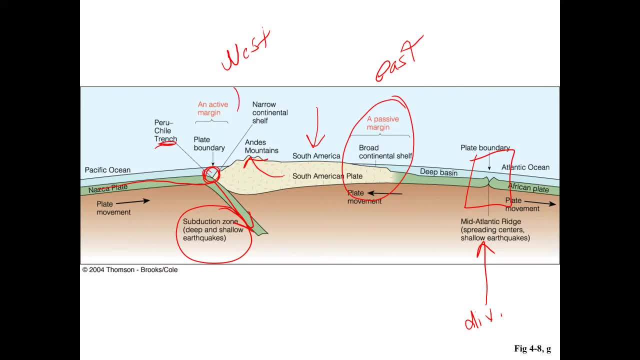 plate is pushing up. So over here in opposition, you have an active boundary. I want to show you one more thing on this figure. Give me one sec On this figure. the next thing that I want to show you is that you have a difference. 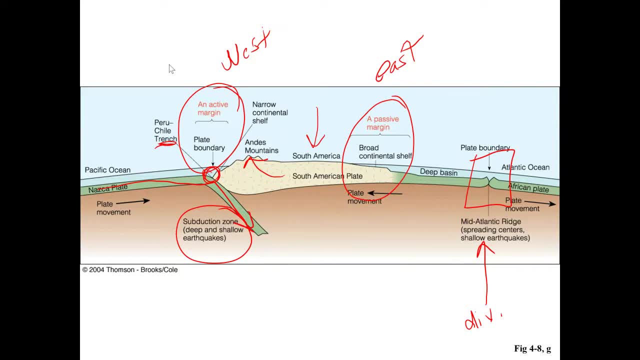 of the actual margin width. okay, Notice how it's called a narrow shelf. The shelf is part of the margin, and here it's called a broad shelf. Again, the shelf is part of the margin. So if you have a on the west side, if you have a convergent boundary, you have an active margin. 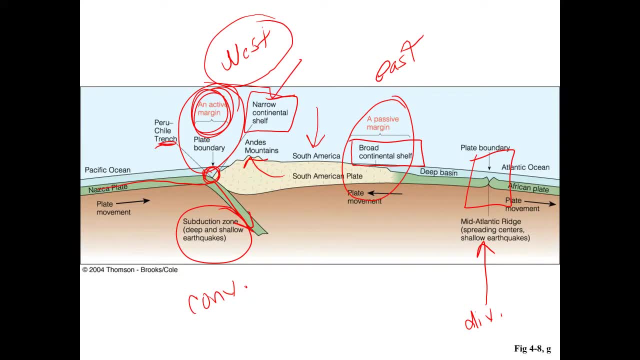 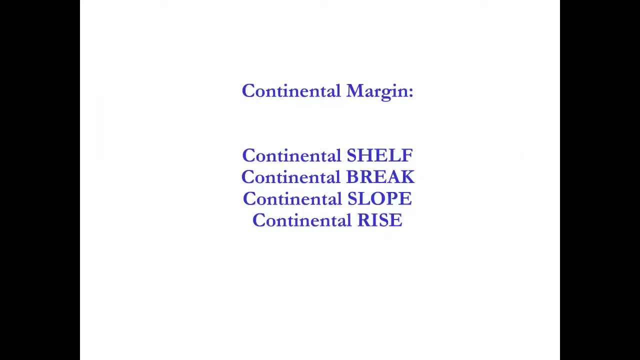 and a narrow shelf. On the opposite side, if you have a divergent boundary, you have a passive margin and a broad shelf. It's a really big distinction. Remember, the four parts of the continental margin are shelf break, slope and rise. 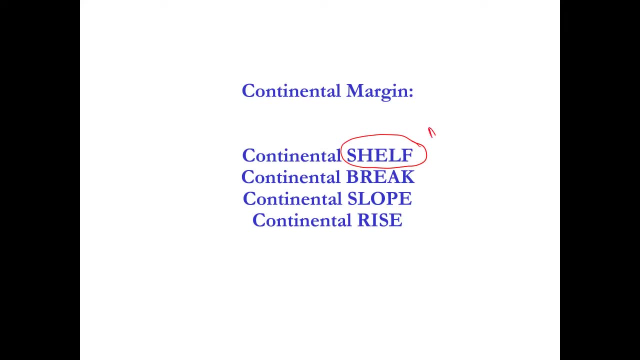 in that order. You're going to look at the shelf. If it's narrow, that's telling you that it's active and that it's part of the margin. You have a convergent boundary near a trench somewhere If, in opposition, that shelf is broad. 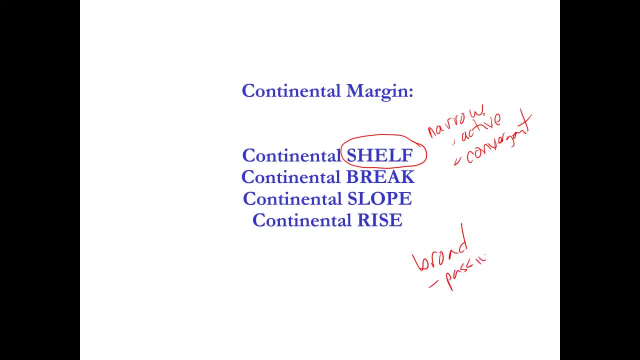 the opposite must happen. You have a passive margin and you're near a divergent boundary. So when you do all of your graphing and mapping and have to label these things, you're going to be able to look at the width of the shelf and look and if it's narrow or broad. 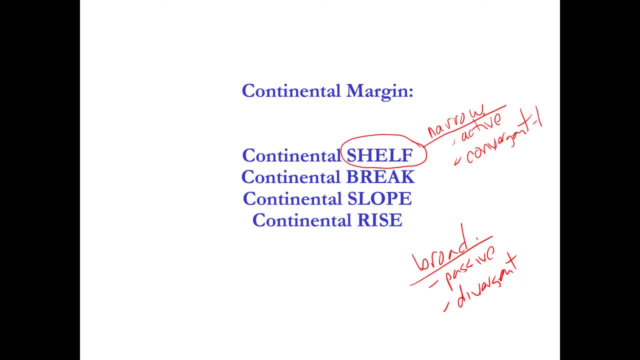 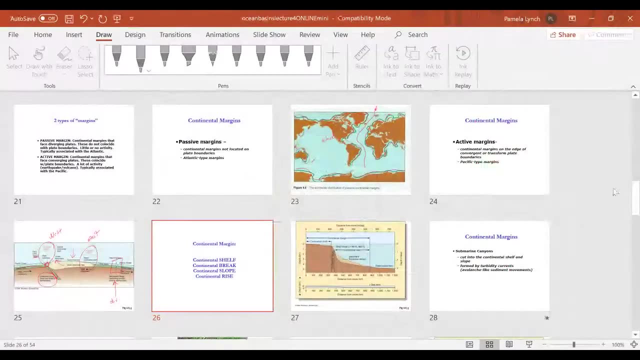 you can tell the difference, in addition, of course, to knowing if it's narrow or broad, If it's near a trench or a mid-ocean system. So the remaining components again, if you're looking at the larger power point, 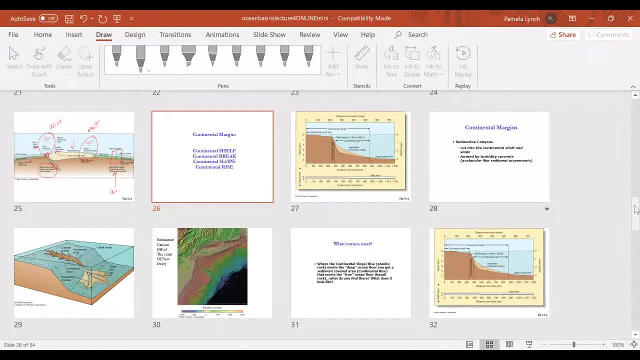 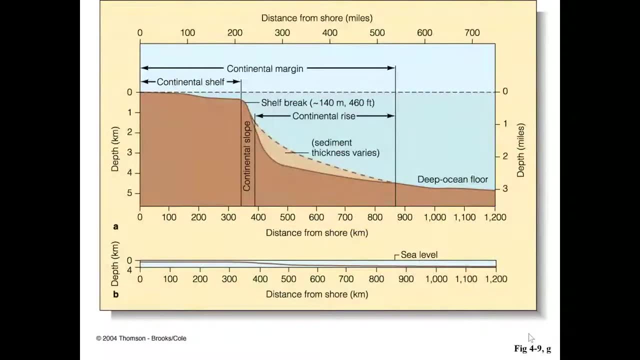 the remaining components here will then give you each text slide of the definitions of the shelf, the break, the slope and the rise Moving on. we've now covered the margin portion In its four components: The shelf, the break, the slope and the rise. 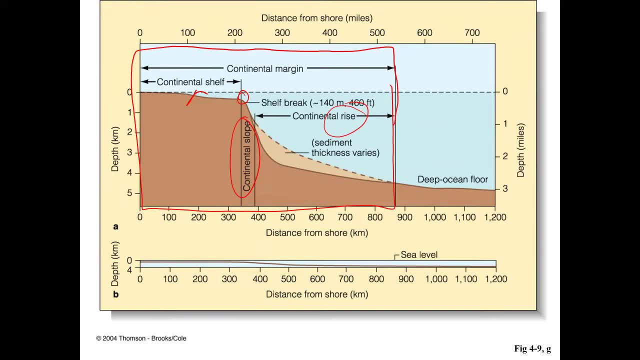 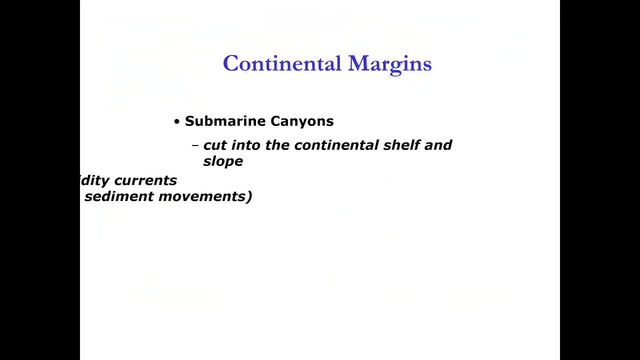 There's one more physical feature that can actually occur in the continental margin that hasn't been mentioned yet. It's called a submarine canyon. Submarine canyon, as it's defined here, is formed by turbidity right. It's sort of like a bunch of sediment coming from higher up and carving out a cut in the shelf and on the slope. 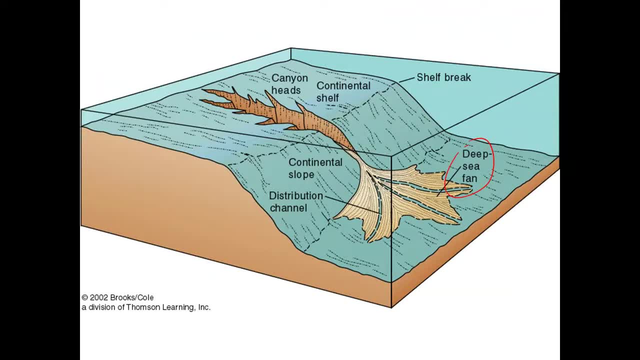 We call it a sea fan at the bottom. Okay, not a sea fan, The marine organism. a sea fan meaning it looks like a bunch of sediment has spread out on the seafloor, And this happens starting at the shelf and going down the slope. 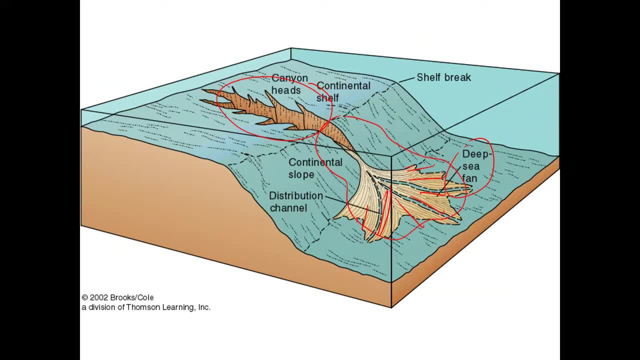 Okay, so this is all part of the margin. still Okay, so this is still going to be continental crust. This happens because there's a rush of water from a river or some sort of upland runoff, carving that canyon out, Our most famous Canyon. you can see it here. 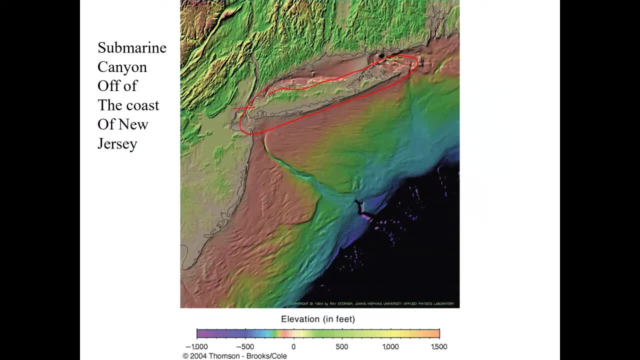 Okay, so here's Long Island. Our most famous Canyon is in New Jersey, So this would have been a level, even continental margin- broad and flat, But there becomes this deep cut right here, right where that submarine canyon is. What this does is it allows deep ocean water and the organisms that are in it, like sharks and big fish, to swim up into that canyon. 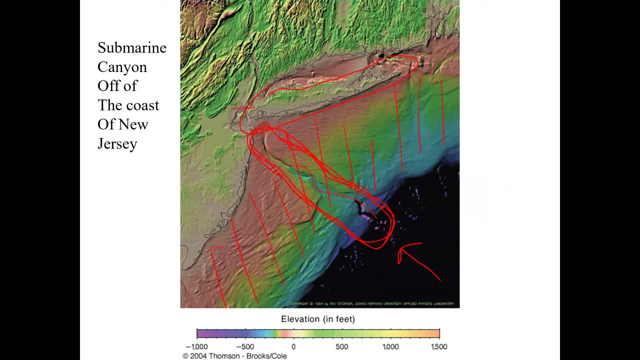 So a lot of people who like to fish love to fish near what we call a submarine canyon. So a lot of people who like to fish love to fish near what we call a submarine canyon. So a lot of people who like to fish love to fish near what we call the canyons because it allows for really good. 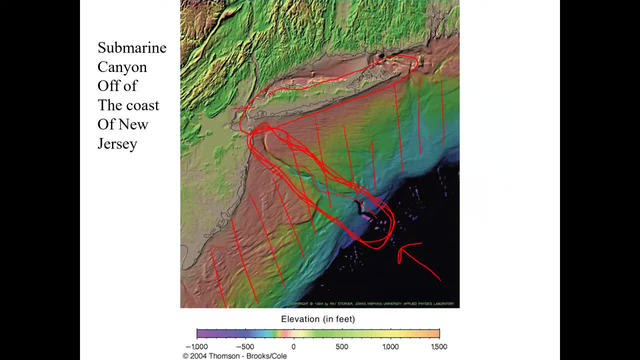 The canyons because it allows for really good sport fishing. Of course, what it does is it just mixes different types of water. because of the different depths in the ocean, The bathymetry changes, which is exactly what this lecture is talking about. 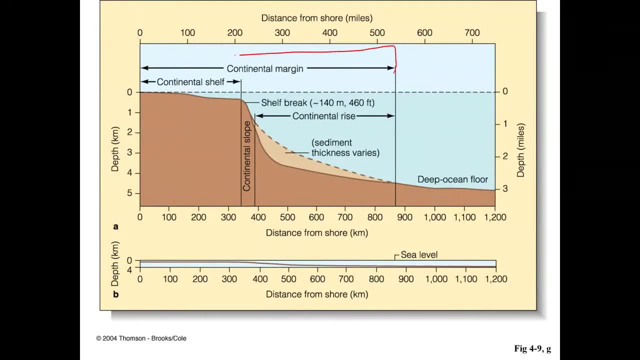 If we move on out from here? okay, so now we've covered five components in the margin: shelf break, slope rise and the one specific example of the submarine Canyon. But what happens if we move outward, out into the deeper ocean? well, we know. first of all, the first thing that happens is we 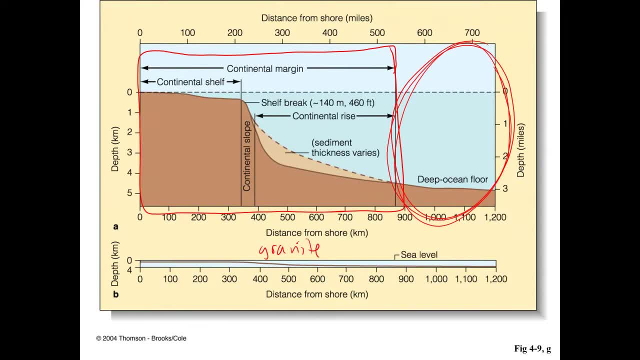 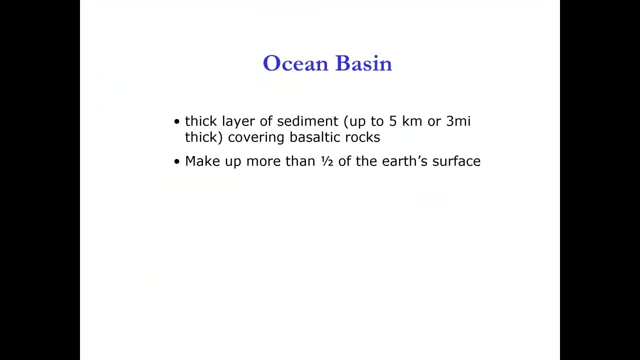 change from granite, which is over here, to basalt. we know we go from older crust to younger crust, but what else happens? well, what's going to happen is: first thing you're going to find is a thick layer of sediment where, essentially, the continental ice meets the basalt rock, which 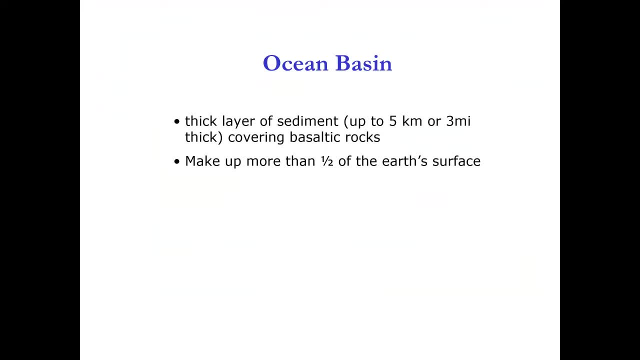 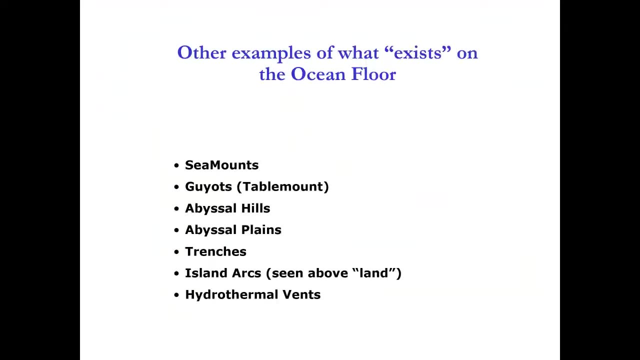 is forming and smashing up against the granite rock at the margin edge. okay, this makes up a huge portion of the earth's surface, more than half- and you're gonna find along that sea floor a whole bunch of features- okay, we call these ocean features now, some of which you already know, right? 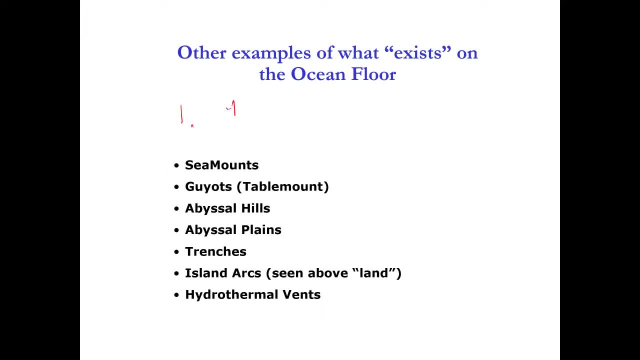 so, first and foremost, this ocean feature that we've talked about is the mid ocean ridge. okay, so we know that that's, of course, in the middle of the sea floor. we've also spoken a lot about trenches. trenches are formed in subduction zones at convergent boundaries. these others, though, other than maybe having 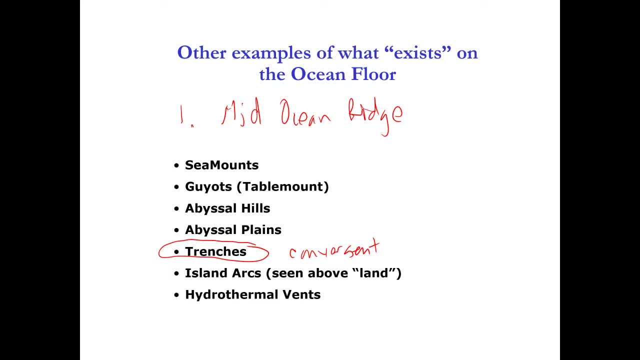 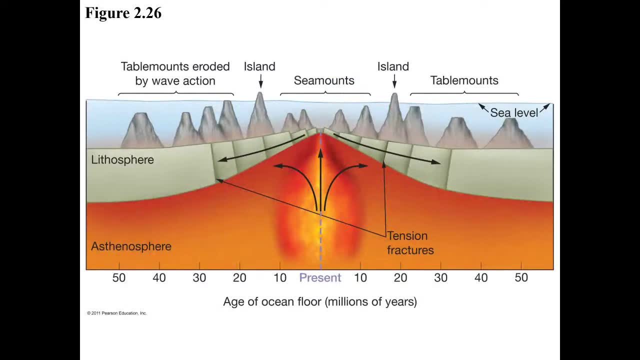 heard about them before, we haven't really spent a lot of focus. so the rest of this lecture is going to go through all of these different features of the sea floor. this particular figure has a couple of examples- okay, two different examples- seamounts and what we call. 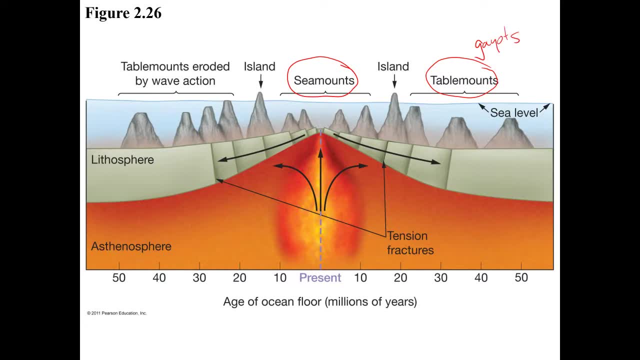 also be called guyutes or gayats- depends again what textbook and what person is talking. they start at the divergent boundary, where sea floor spreading is and a seamount- okay- is submerged, so it has to be under the water and pointy, as opposed to a table mount, which is also submerged. 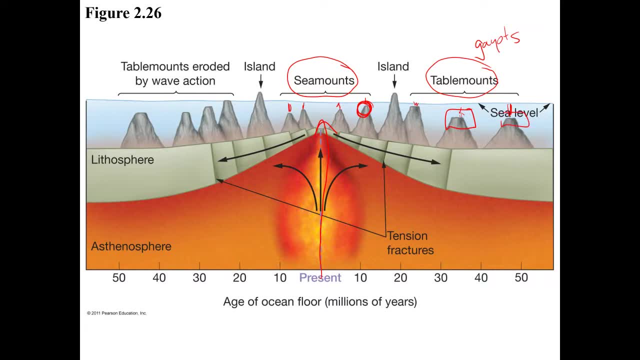 but it's flat. so they're literally just submerged portions of the ocean, basin crust, basalt crust- that are under the water and either pointy or flat. a seat mount has a pointy tip and a table mount has a flat tip- the only other evidence that you see here. 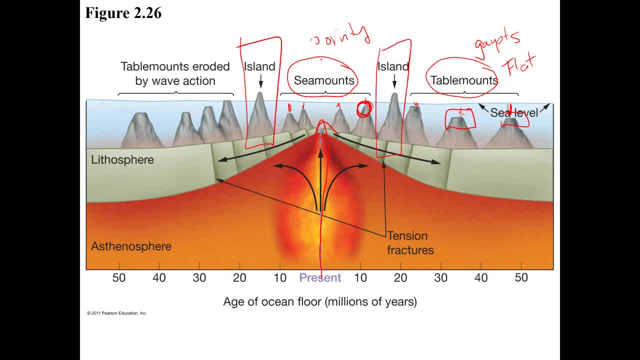 are things above sea level. we already know what those are, right, anything above sea level we call an island. over time, though, if that island gets pushed away- because, remember, these plates are shifting to the left and to the right, so as that island moves further and further over the years, 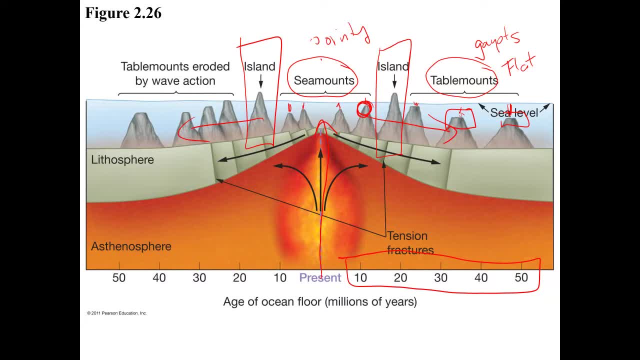 it will eventually sink. so we talk about, for example, the lost city of atlantis. right, there could have been an island up above the sea level and was habitable, and over time, millions of years, it sunk, which then made it inhabitable, for humans at least, and they then become, after an island, they become a sea level and then they become an island. 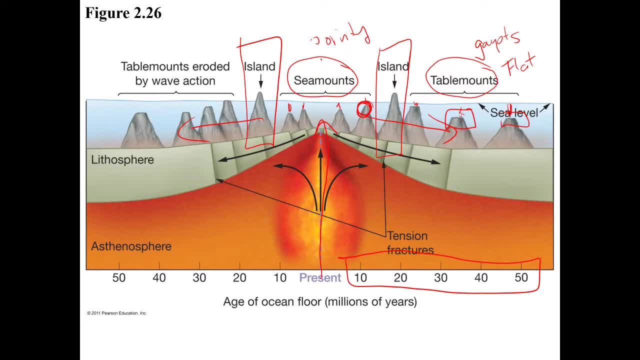 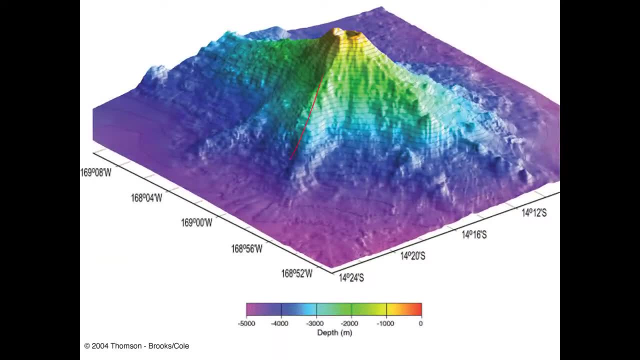 a seamount and then it erodes away like getting a flat top haircut. it erodes away and becomes a table mount. even further away than that, of course, you're going to have to go down in depth and down in elevation, right going down an island. what actually happens on these outer edges? well, 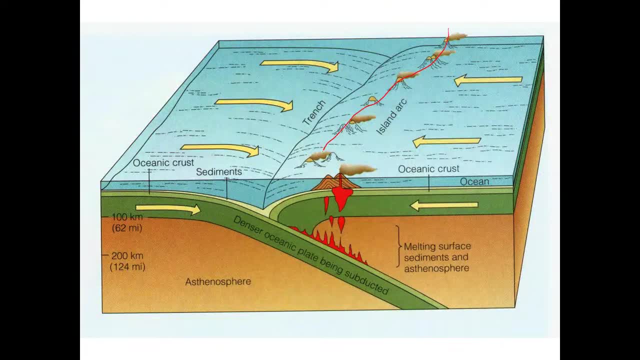 you're going to find that you're going to have that original island system. if you were to look under the water here, you would find seamounts and table mounts in these areas not exposed again because they'd be below sea level and on the opposite side. what are you finding in this big, vast expanse? 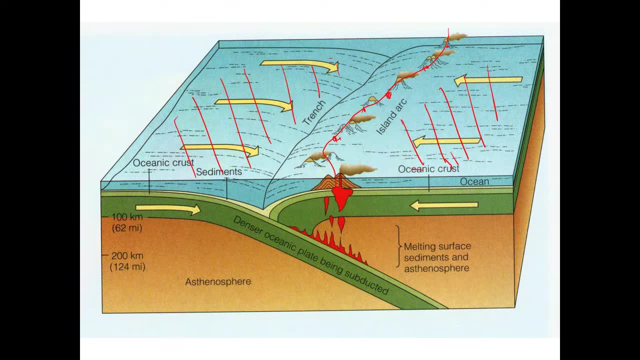 that's the rest of what the ocean basins are going to cover. so, in other words, an island arc is the highest, tallest component, followed next by a seamount getting deeper in the ocean right, less tall, followed by a table mount even deeper in the ocean and even less tall, followed, of course, by the abyssal hills and the abyssal plains. 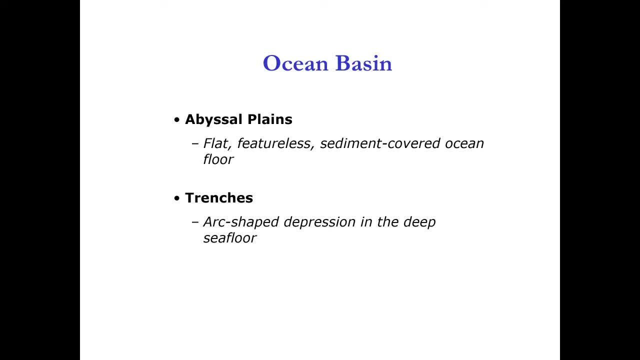 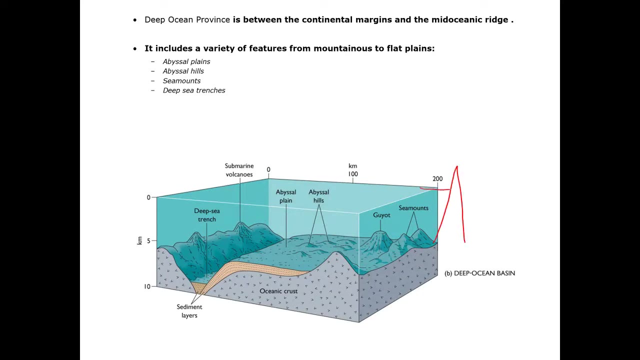 these are going to surround those trenches. those trenches are going to be at the edge of where the plate boundary meets. okay, now, at that exact same location, of course, you're going to have to find what's left. so imagine that an island is here again above sea level when that erodes away and 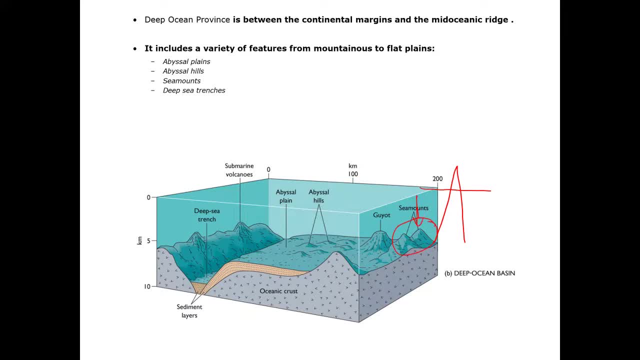 moves further away, you get a seamount submerged, but taller. when that erodes away, you get a table mount or a guy. you even deeper down. you get a table mount or a guy. you even deeper down and flatter. remove that away and you get abyssal hills and abyssal plains. abyssal hills are just. 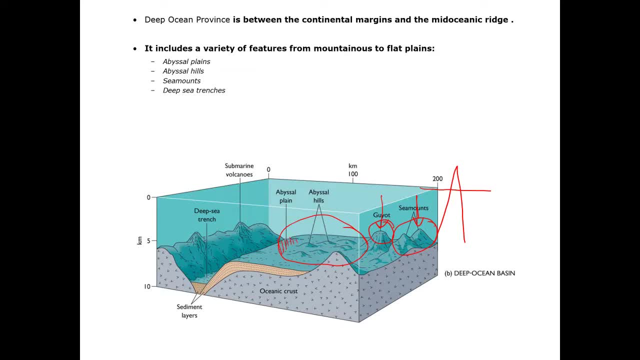 slightly higher than the plane, which is the deepest part of the ocean. we call that the flat, featureless portion of the ocean. those are all components of literally the oceanic crust. remember other components of the oceanic crust can always be trenches and mid-ocean ridge systems on. 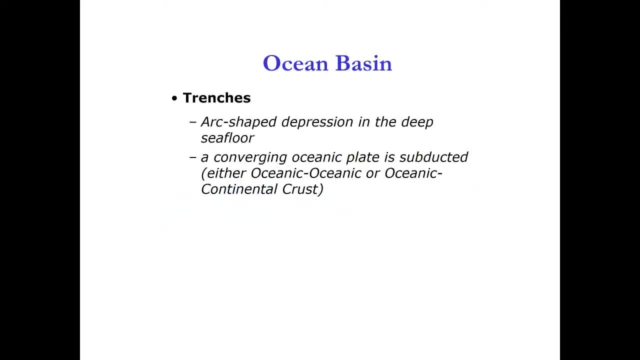 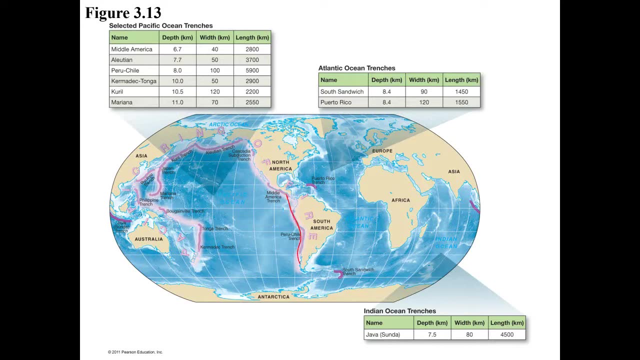 the opposite side of the ocean, which is what we're going to talk about next. So let's get started decide where a dive boundary would be If you follow the trench line. remember, these are active margins. So if you follow that trench line, it makes sense that those active margins follow that. 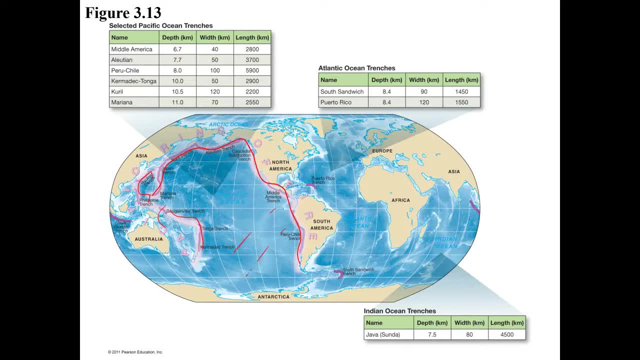 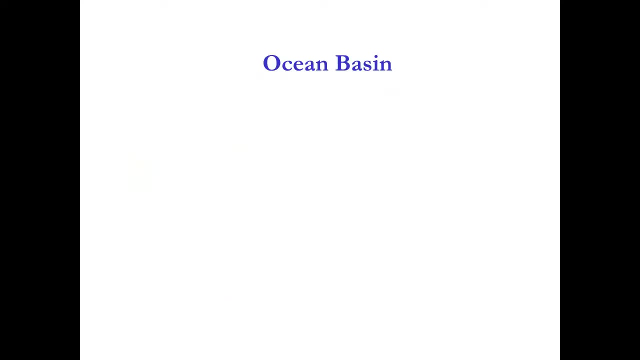 same location. We can then assume that in this portion of the ocean, you're going to find your islands, your mounts, your table mounts, your abyssal hills and your abyssal plains- Another visual of the same thing. Finally, our last feature. Now, I'm a marine biologist. I also teach oceanography, of course. 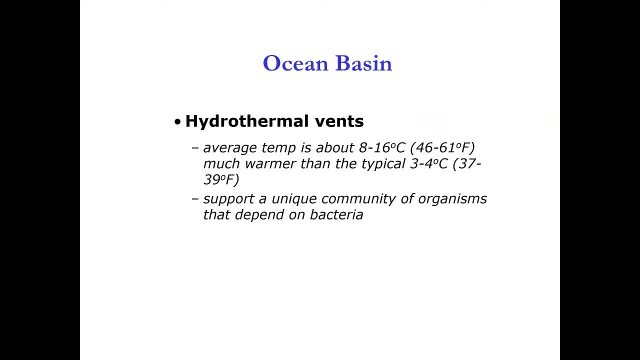 and knowing marine biology sort of goes hand in hand with oceanography. But from a marine biological perspective the most fascinating part of this entire lecture is that in the part of the ocean that you would think is the deepest, darkest, sky-high and the most beautiful part of the 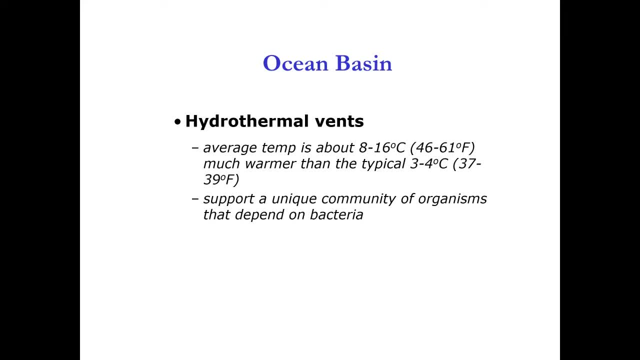 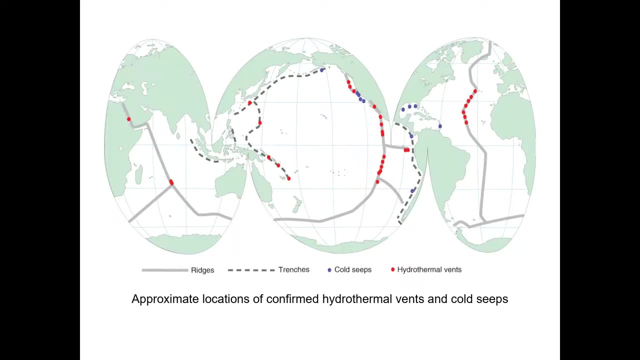 ocean, the most mysterious, hardest to live, we find a true thriving biological community. It's called a hydrothermal vent, hydro water, thermal temperature vent opening. These occur at the exact same location that the mid-ocean ridge systems are. So again, here's our mid-Atlantic ridge. 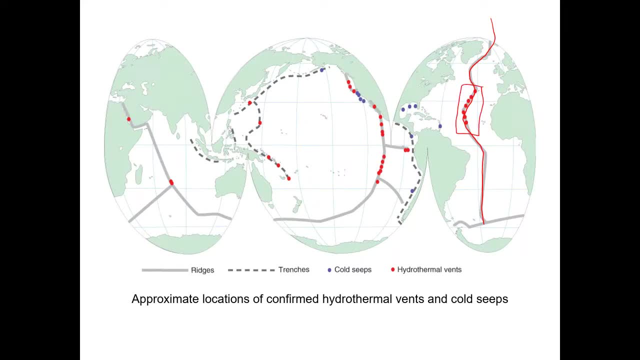 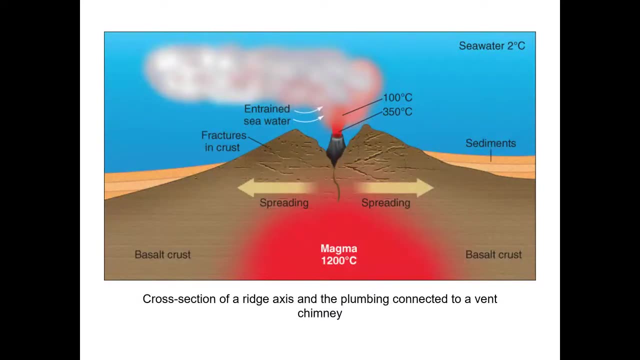 And sure enough, we have a series of thermal vents that have been discovered all along the center of that ridge line. They are a true thriving biological community, And so we're going to go ahead and take a look at that. So we have a true community of a collection of material that can 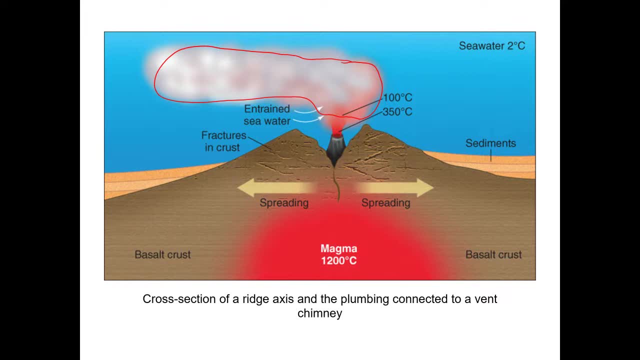 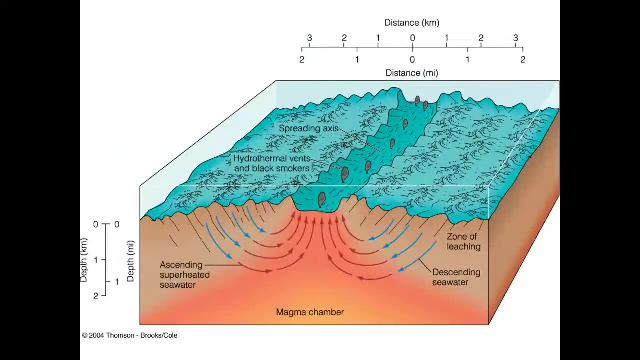 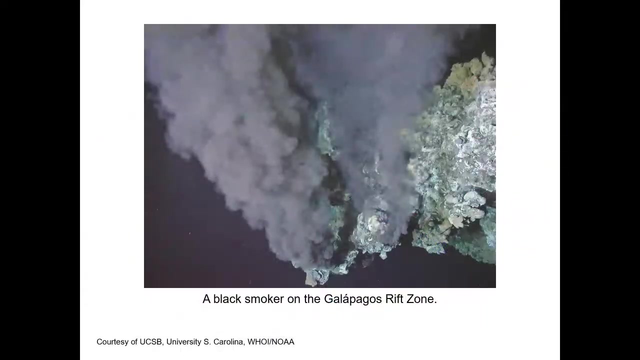 serve as food. so chemicals, essentially, that can serve as food at the spreading center And along this chimney or this volcano or vent, we actually end up with food sources, chemical food sources for marine organisms. Those marine organisms can feed off that smoke which again is filled with. 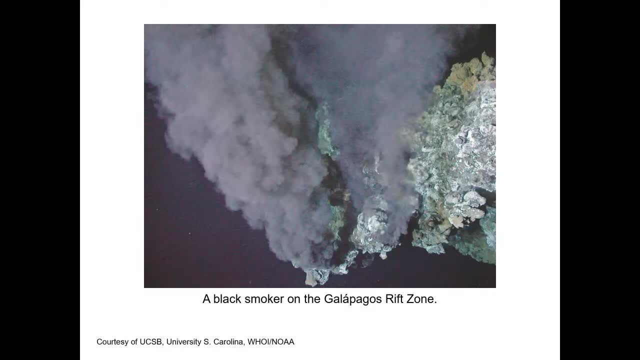 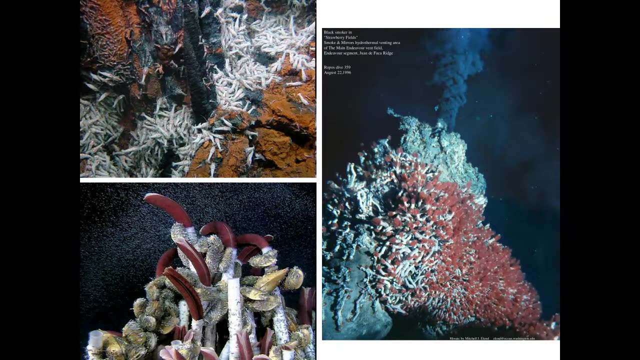 chemicals and elements, minerals, And that can feed off that smoke, which again is filled with chemical material that can be synthesized, through something called chemosynthesis, by marine organisms that can literally cement themselves on the vent. So this would be the opening of the 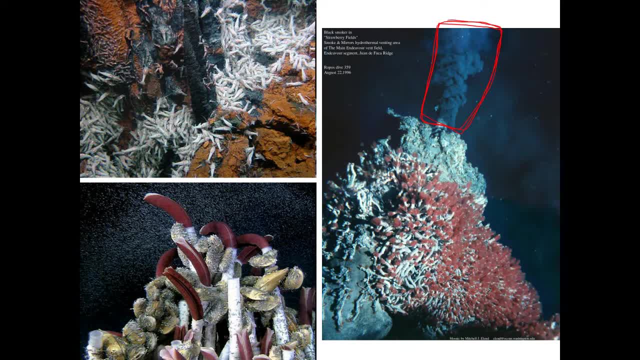 mid-ocean ridge system. There's the smoke or the material coming from the asthenosphere. If this were above the water on an island, that would look red like lava. okay, It's because it's so cold here, but the material that's coming out of the vent is so hot that it precipitates into what looks like. 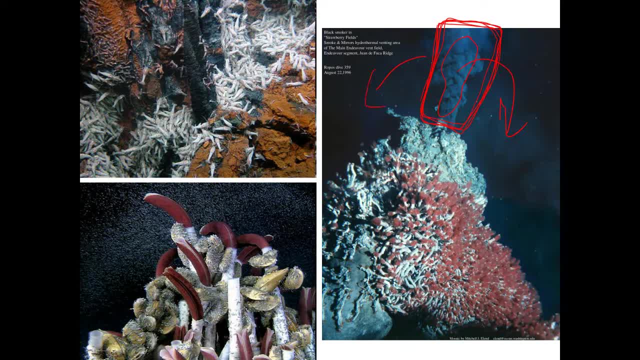 a black cloud, But this black cloud can actually rain down chemicals which serve as food for all of these marine organisms. Now here we're showing you tube worms, which is probably the most popular and famous of all of the marine vent communities. There's a close-up: These are called Pompeii worms. 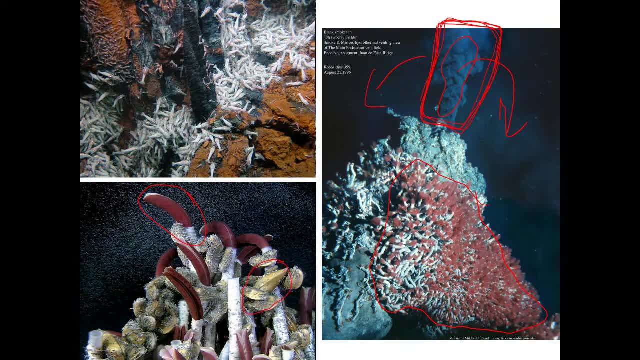 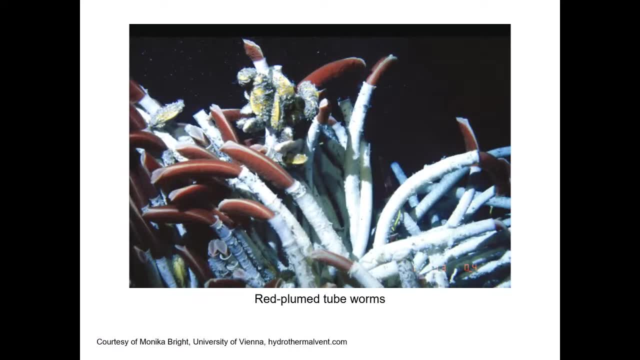 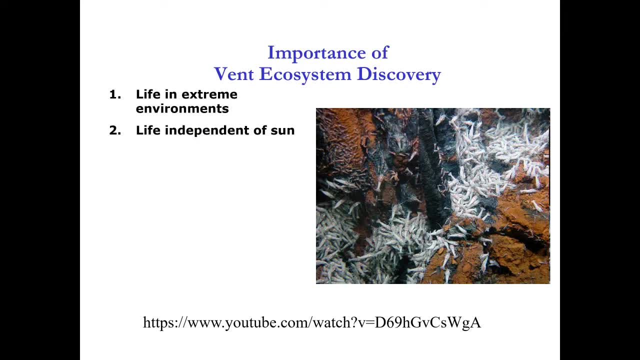 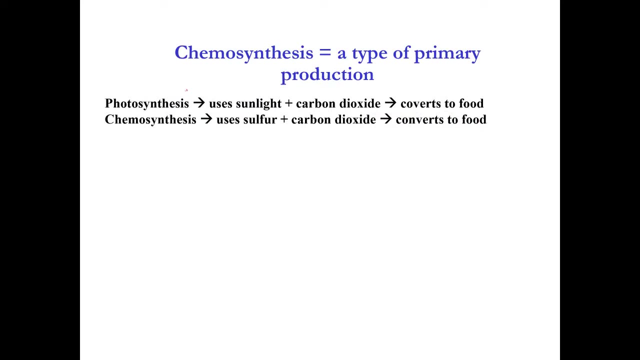 them, but we have a lot of different kinds of worms here, Okay, so let's look at the continuous. How many of these did we get? How many did we get? But instead of having sunlight, we use chemicals. In this particular example, sulfur is the chemical. 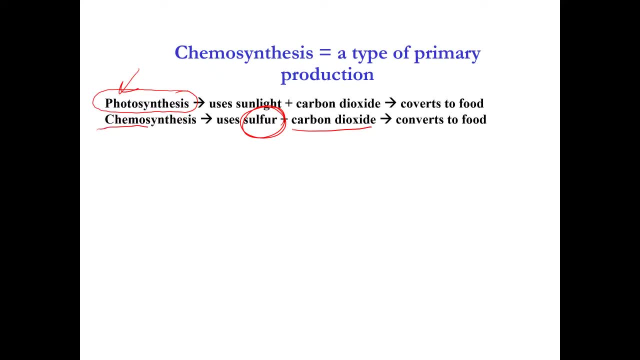 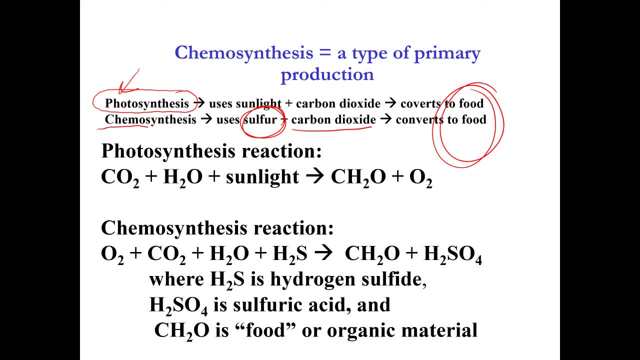 So, instead of synthesizing light, you synthesize chemicals. Either way, you're making a food source And those marine organisms are going through a process that is the exact opposite of photosynthesis. So in photosynthesis, we take in dioxide- cleaning our planet, of course- and we produce oxygen. 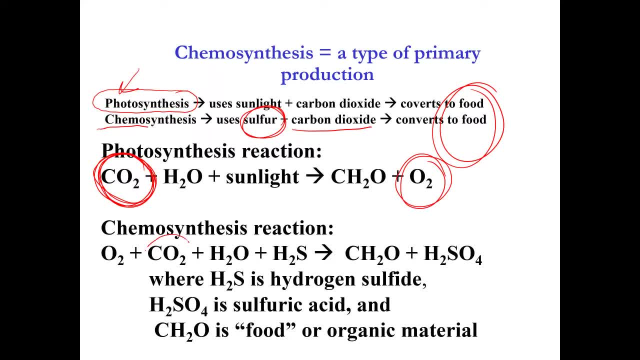 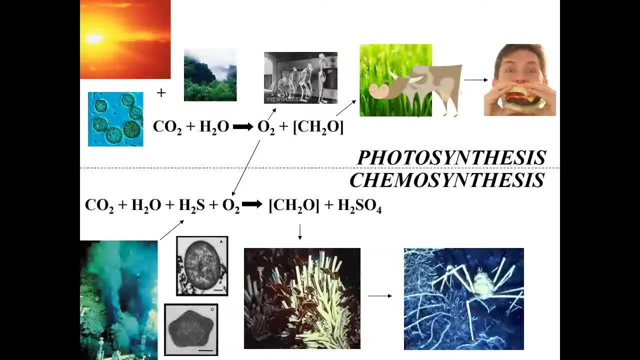 In chemosynthesis you still have carbon dioxide, but we also use oxygen plus some sort of chemical material And we produce hydrogen sulfide, sulfuric acid and the food source for the organisms to live from. So you've taken essentially an inhospitable, an inhabitable location: the deepest, darkest, highest pressure. 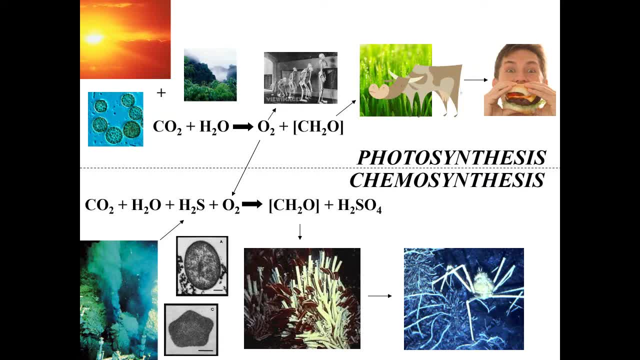 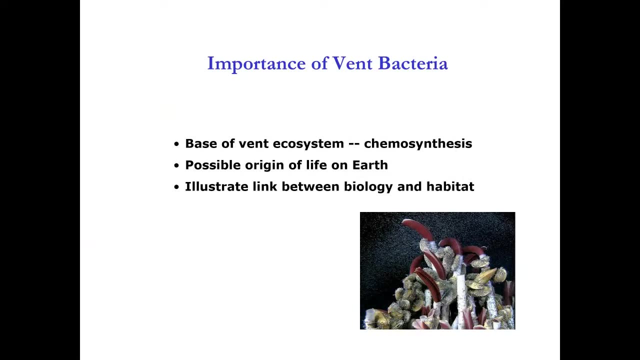 most most likely to be named location, that you would find nothing living in the planet And you have a huge diversity of marine organisms. We believe that the importance of the vent bacteria which live inside the gut cavities, a lot of these marine organisms that allow them to chemosynthesize chemicals. 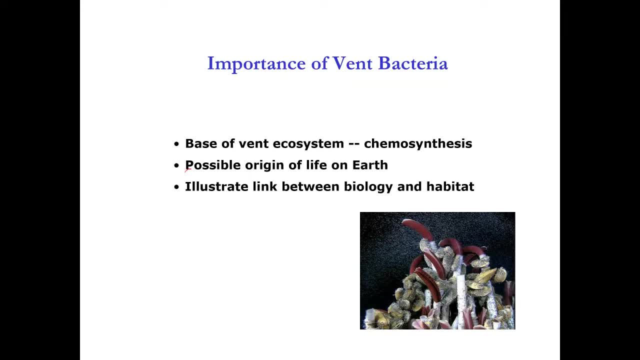 The importance of that vent. bacteria may link back to the possible origins of life. Archaea. extremophiles right. Organisms that, Organisms that are four million, excuse me, four billion years old. pretty, pretty, pretty crazy. 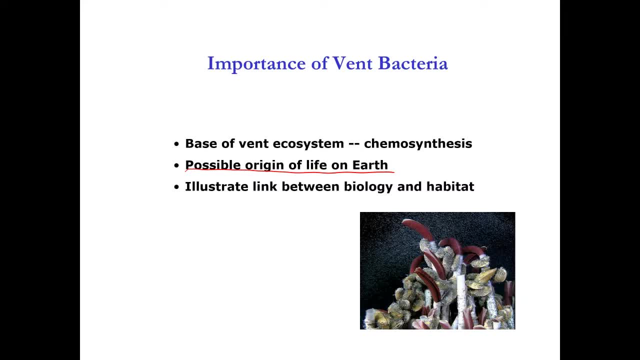 If you're into this sort of thing, you want to make sure that you take a marine biology class in the spring or whenever you're available. We spend a lot of time talking about specific marine bacteria and bacteria as a whole and their importance in the marine community, as well as looking at hydrothermal organisms and deep sea organisms. 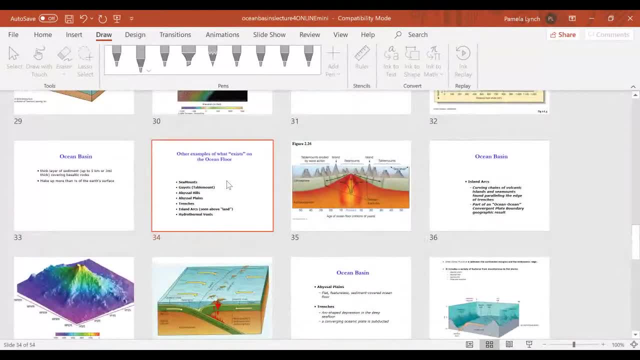 So, just to summarize, I want to cover the second half of this lecture one more time. Make sure that you understand what we've talked about. So just to summarize, I want to cover the second half of this lecture one more time. Make sure that you understand what we've talked about.